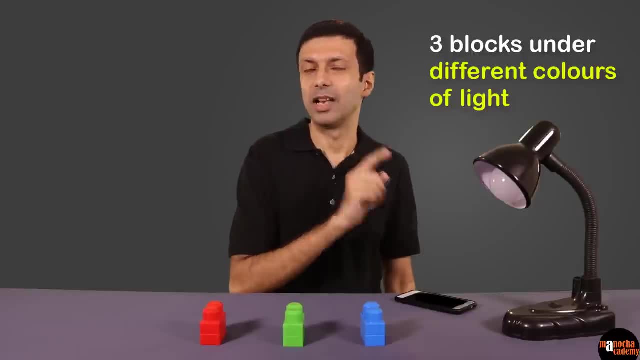 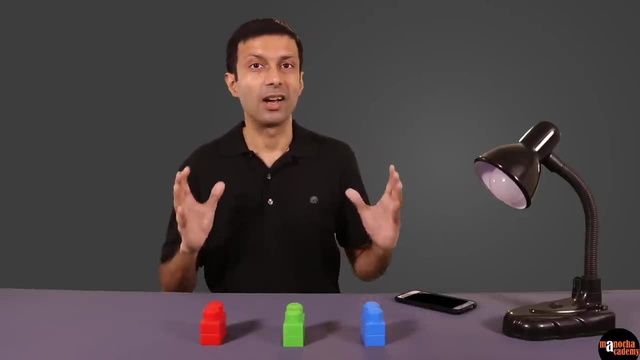 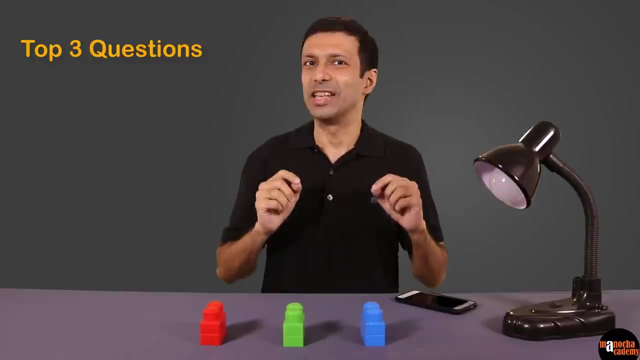 And we are going to look at these three blocks under different colors of light- Red light, green light and blue light- And let's see what these blocks look like under colored light. And, as usual, we'll finish off with our top three questions on this topic. 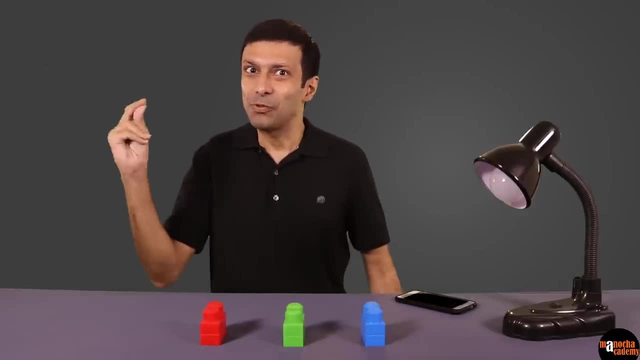 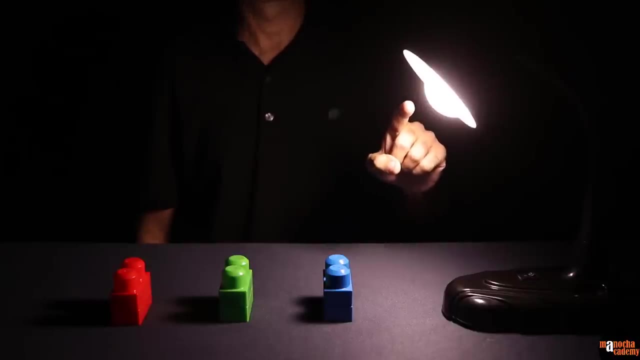 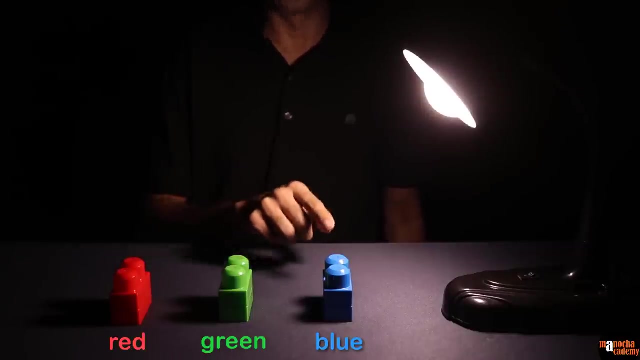 So are you ready for our exciting experiment? Lights off, please. I'm now going to turn on our magic bulb First. as you can see, the bulb is giving off white light. We have three blocks here: Red, green and blue. 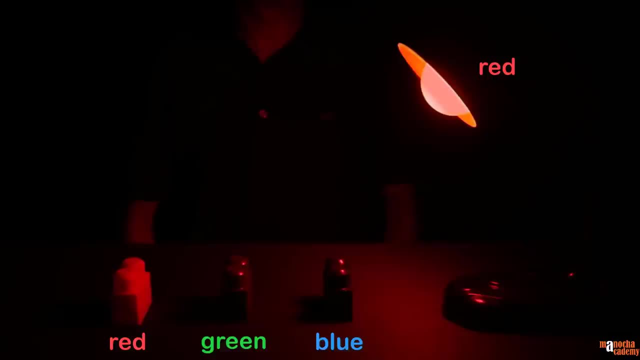 Now I'm going to change the color of the bulb to red. Wow, Can you see the red block here? But we can't recognize the color of the other two blocks. They appear blackish. This is in fact the green block and this is the blue block. 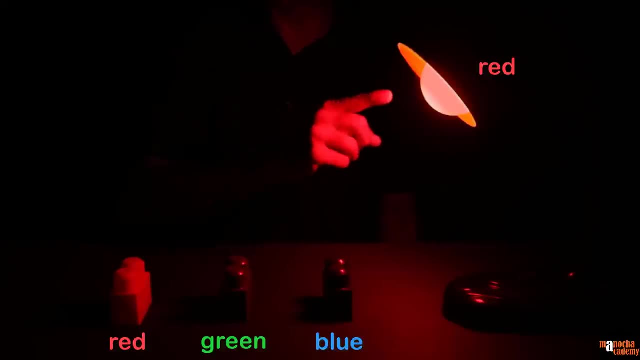 Now why is this happening? Because there's only red light here And the red block is able to reflect the red light, so it's visible and appears red in color, But the green block absorbs all the red light and has no light to reflect. 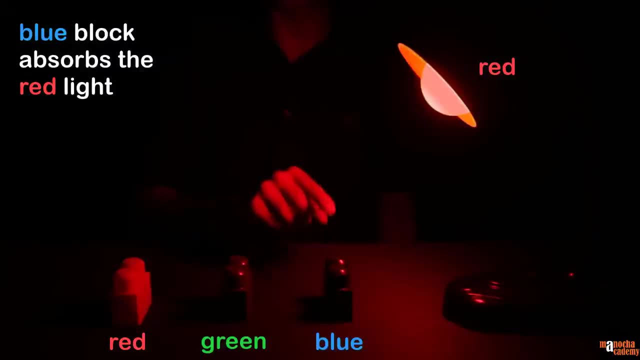 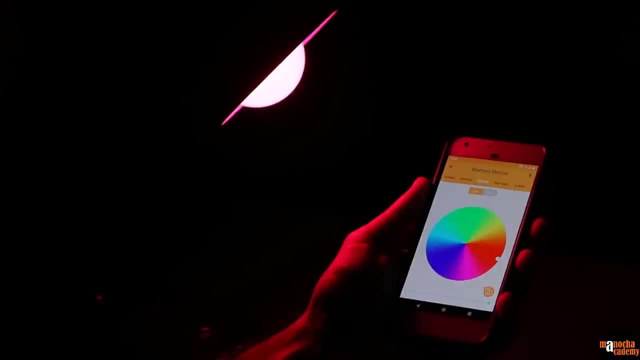 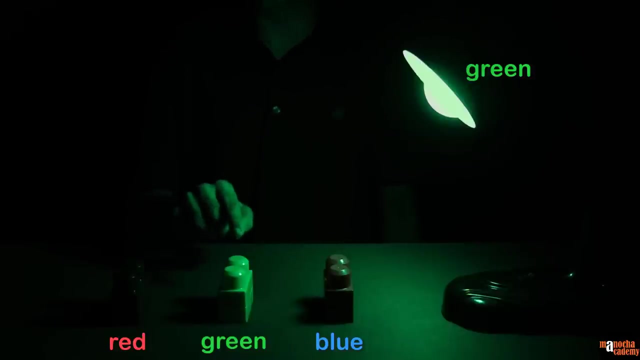 So it appears black, And same is the case with the blue block. It absorbs the red light and hence appears blackish in color. Now I'm going to change the color of the bulb to green. Under green light can you see that the green block is visible? 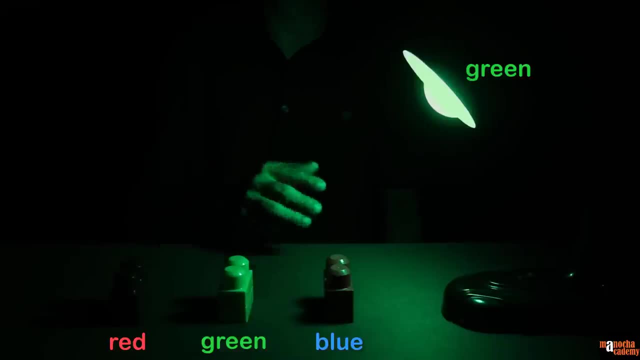 But the red block and the blue block appear blackish in color Because the green block is reflecting all the green light, But the red block and the blue block are visible, But the red block and the blue block are not. But the red block and the blue block absorb the green light. 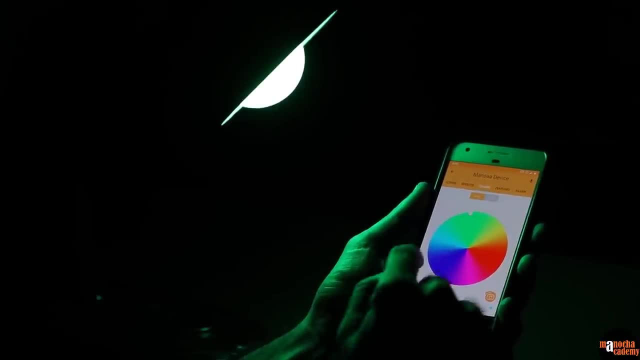 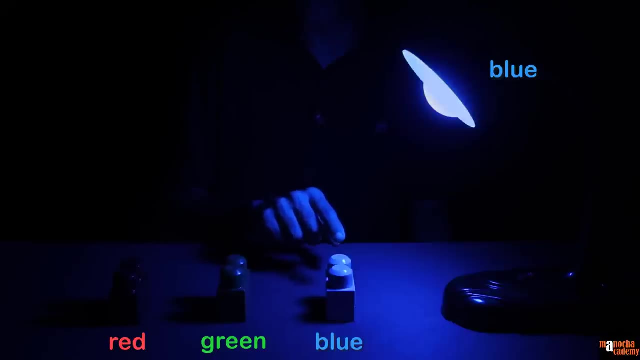 Hence they appear blackish. Now I'm going to change the color of the bulb to blue. Now what do we have here under blue light? Can you see that the blue block is now visible, But the green and red block appear dark or black in color? 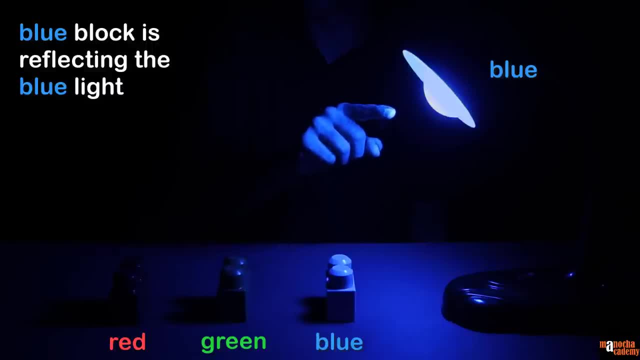 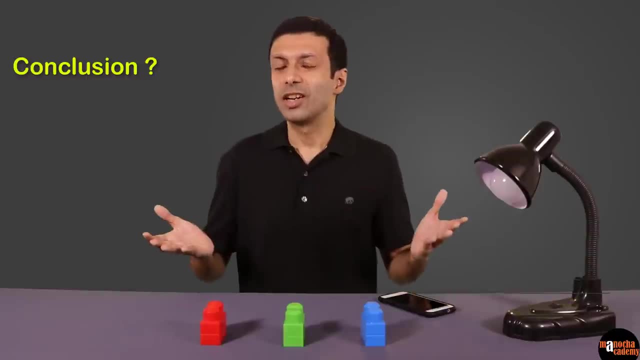 Because the blue block is reflecting all of the blue light, But the green and red block are absorbing the blue light and hence they appear black in color. So what's our conclusion from the experiment? An object reflects light that matches the color of the object. 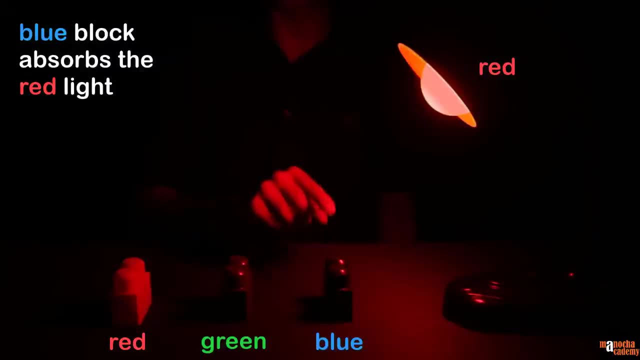 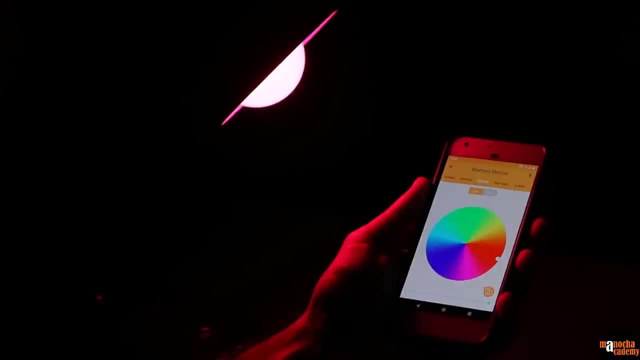 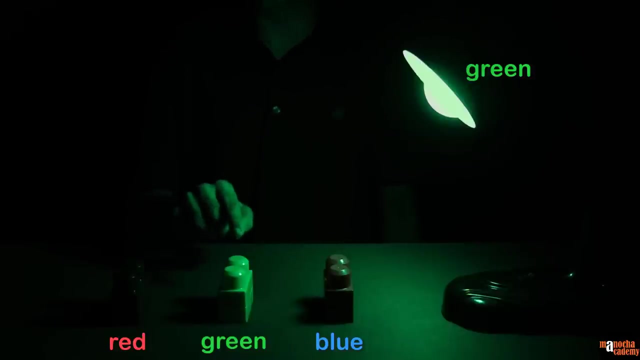 So it appears black, And same is the case with the blue block. It absorbs the red light and hence appears blackish in color. Now I'm going to change the color of the bulb to green. Under green light can you see that the green block is visible? 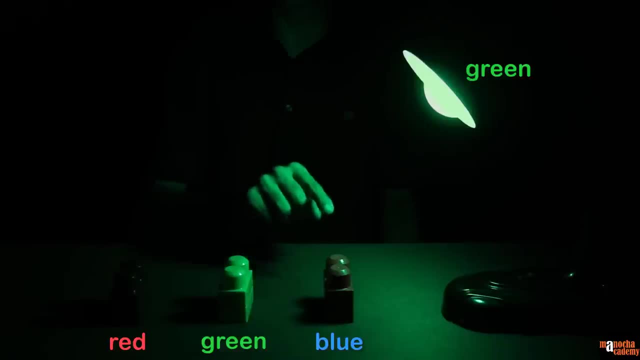 But the red block and the blue block appear blackish in color Because the green block is reflecting all the green light, But the red block and the blue block are visible. But the red block and the blue block appear blackish in color Because the green block is visible. 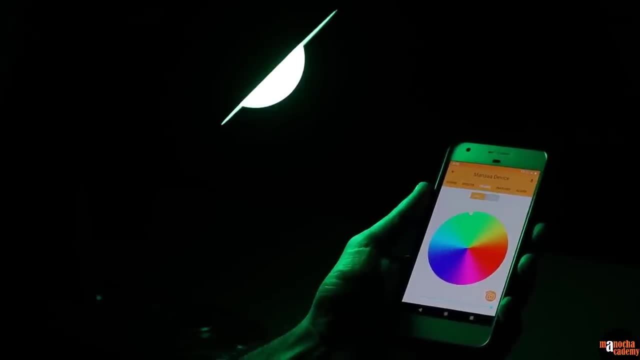 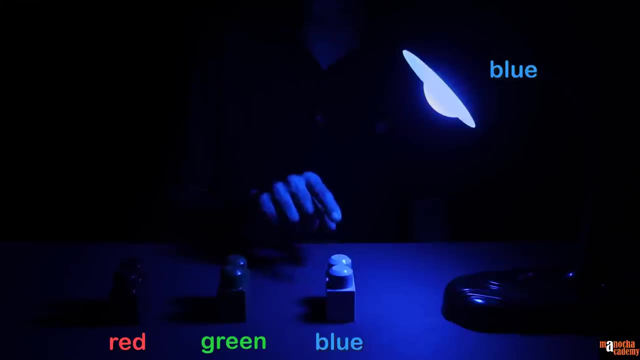 But the red block is visible. Now I'm going to change the color of the bulb to blue. Now what do we have here under blue light? Can you see that the blue block is now visible, But the green and red block appear dark or black in color? 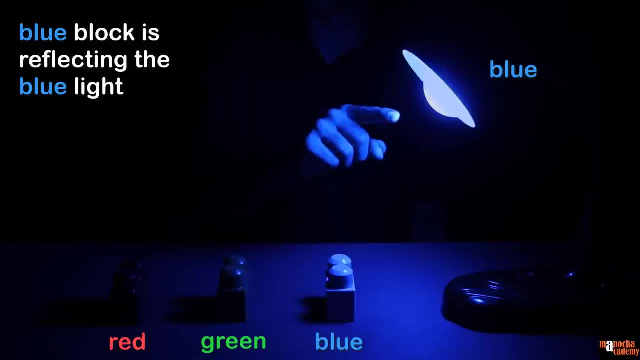 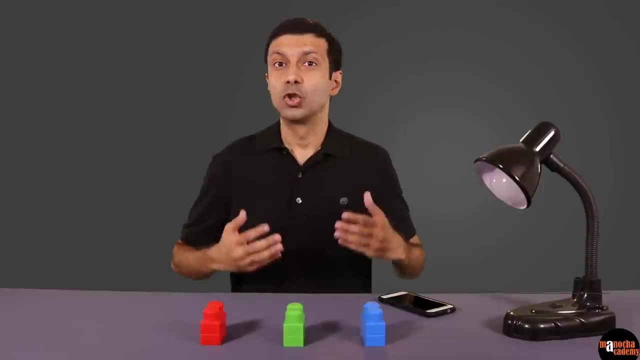 Because the blue block is reflecting all the blue light, But the green and red block are absorbing the blue light and hence they appear black in color. So what's our conclusion from the experiment? Conclusion from the experiment: an object reflects light that matches the color of the. 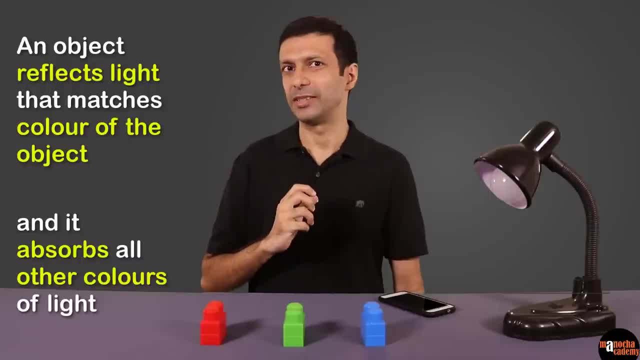 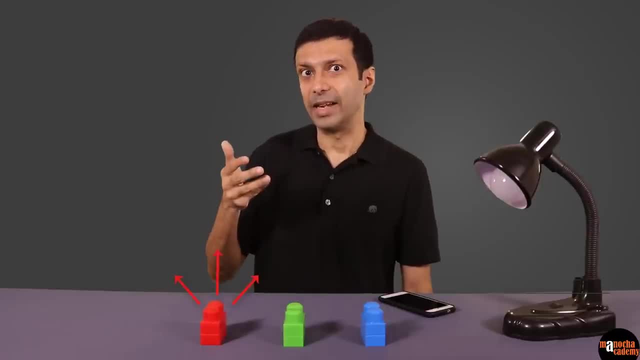 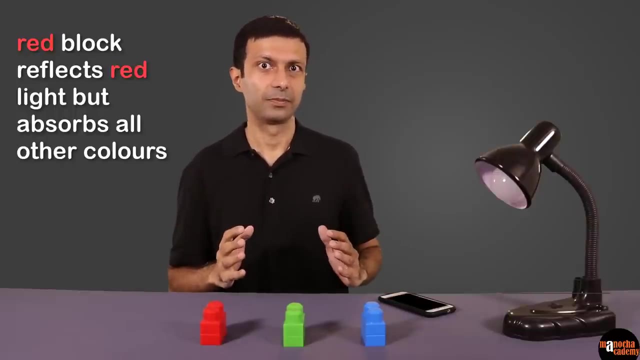 object and it absorbs all other colors of light. Let's take an example. If we consider this red block here, it's reflecting red light. That's why it appears red to us, But it's absorbing all the other colors of light. Now, when this red block was placed under different colored light, what did it look like? 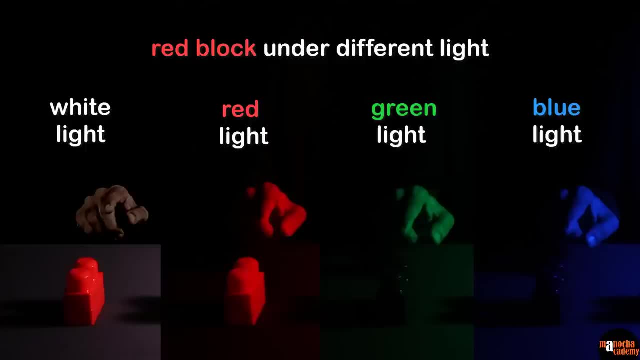 So under red color it looked red in color, But when placed in blue and green light it looked black, because it was absorbing the green and blue light and it was not able to reflect any light because it can only reflect red light. That's why it appeared black. 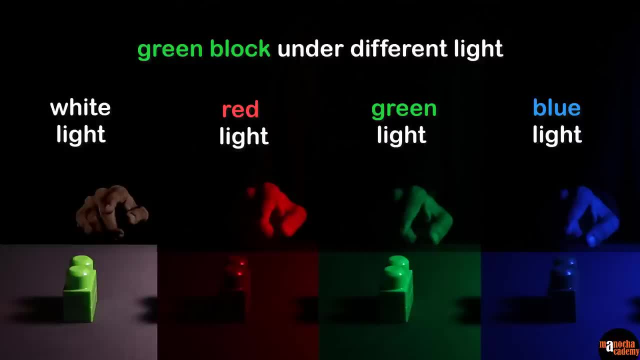 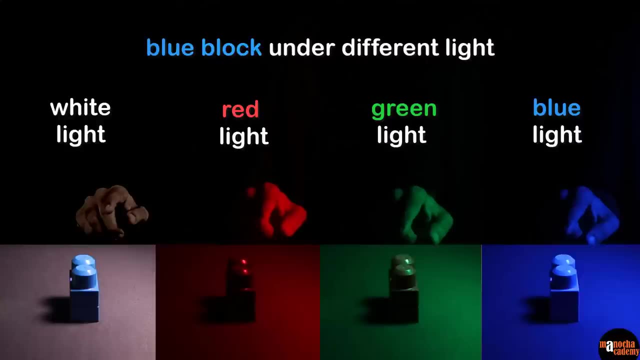 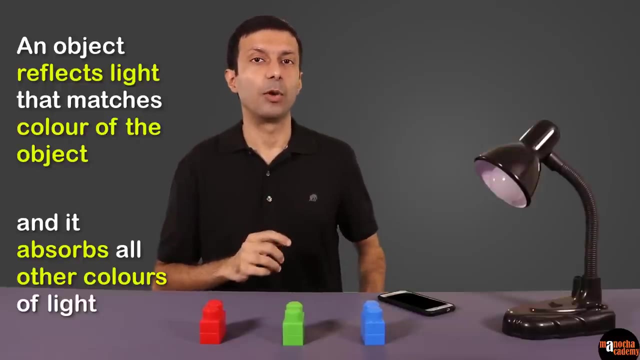 Similarly, the green block was visible under green light, but appeared blackish under red and blue light, And same is the case for the blue block. So clearly we can see that these objects are reflecting light of their color, but they are absorbing all the other colors. 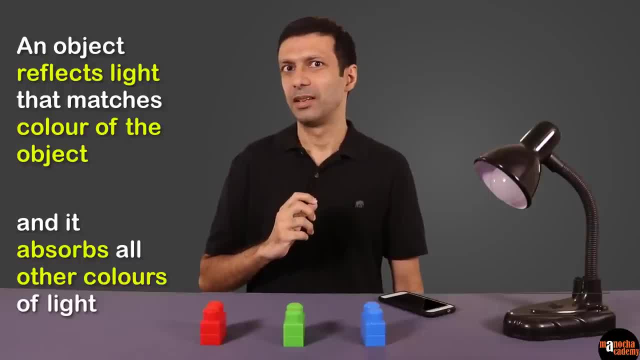 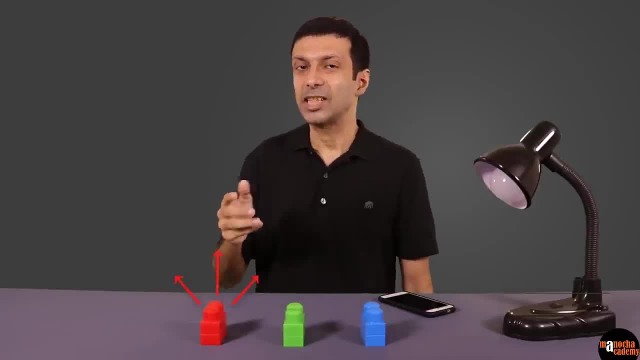 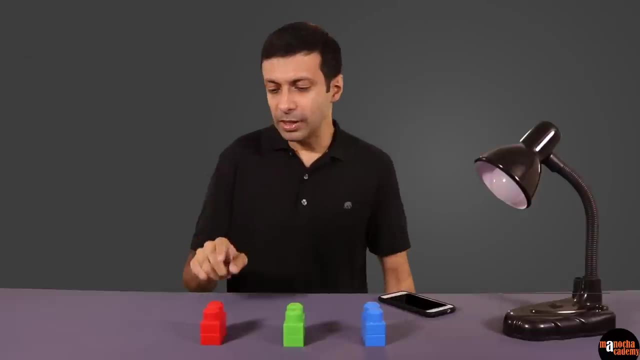 And it absorbs all other colors of light. Let's take an example. If we consider this red block here, it's reflecting red light. That's why it appears red to us, But it's absorbing all the other colors of light. Now, when this red block was placed under different colored light, 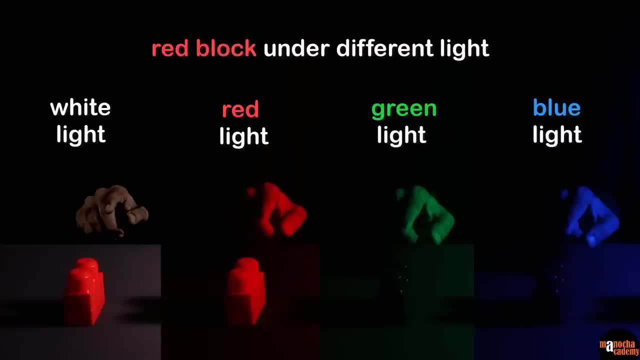 what did it look like? So under red color it looked red in color, But when placed in blue and green light it looked black Because it was absorbing the green and blue light and it was not able to reflect any light, Because it can only reflect red light. 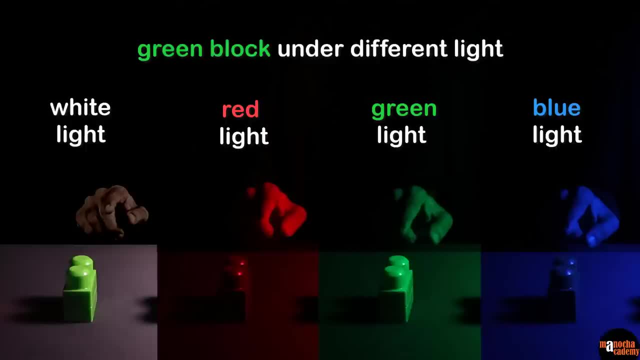 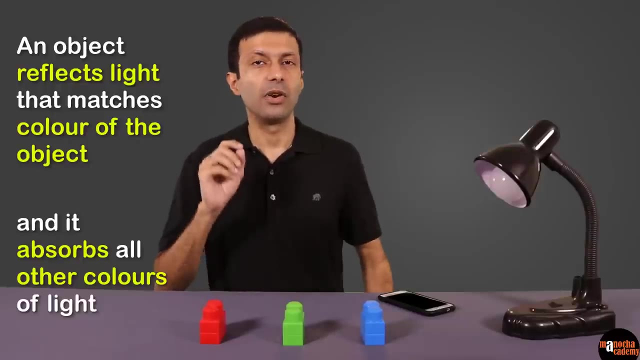 That's why it appeared black. Similarly, the green block was visible under green light, but appeared blackish under red and blue light, And same is the case for the blue block. So clearly we can see that these objects are reflecting light of their color, but they are absorbing all the other colors. 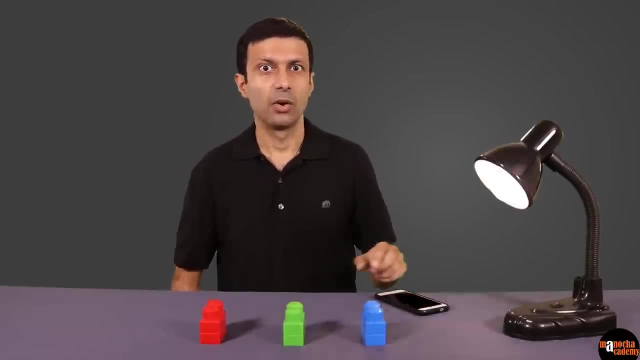 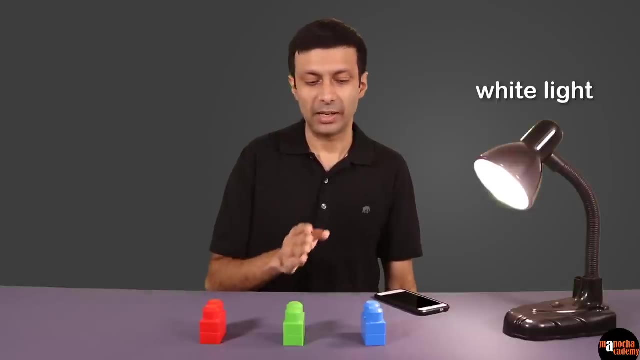 When we look at these three blocks under white light- whether it's coming from this bulb or from the lights in this room- we can see all the three colors: red, green and blue. The red block is reflecting red light. The green block reflects green light. 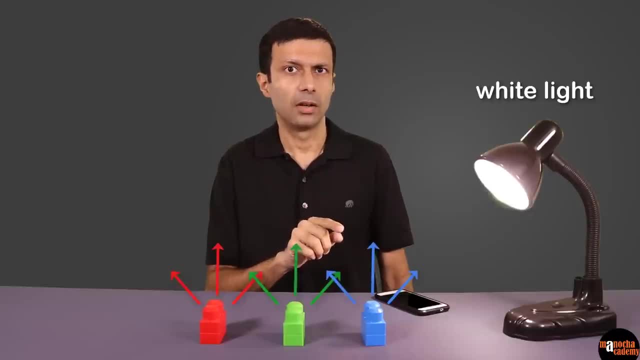 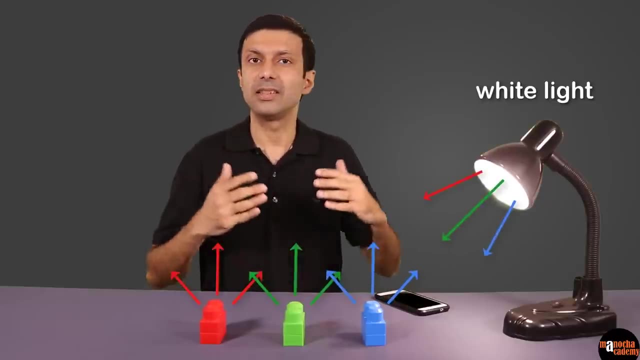 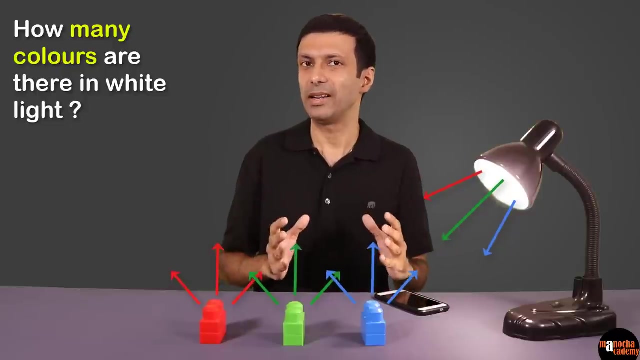 And the blue block reflects blue light. So what does this tell us about white light? White light is actually not white. It at least contains these three colors: red, green and blue. But do you know how many colors there are actually in white light? 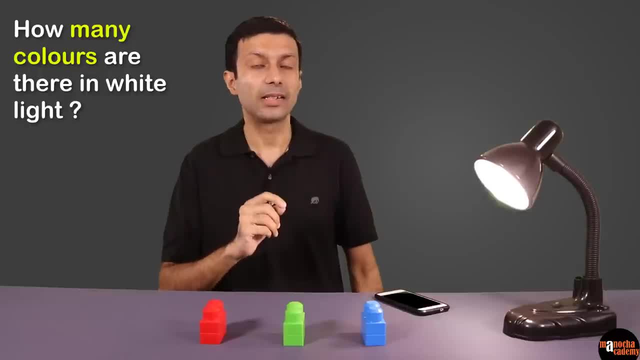 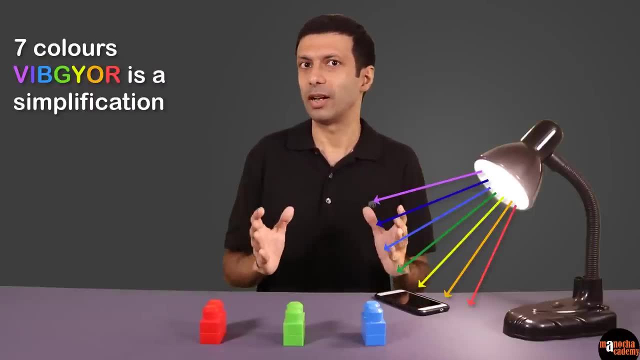 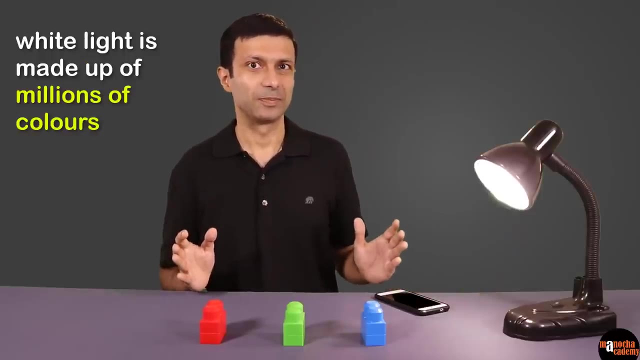 That's right. the correct answer is: white light contains millions and millions of colors. You may have heard of the seven rainbow colors or the Vibhya colors, but that's just a simplification. White light is made up of millions and millions of colors. 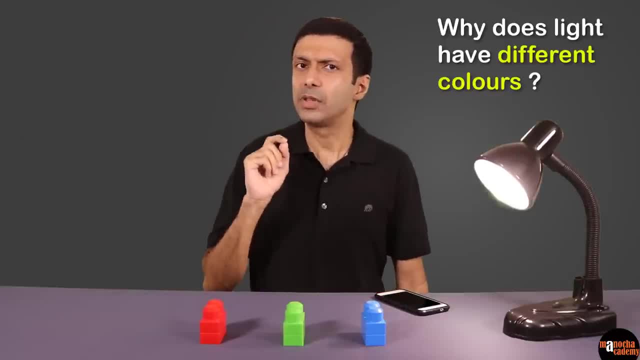 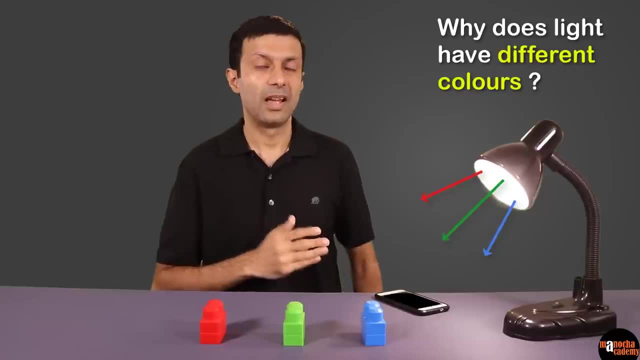 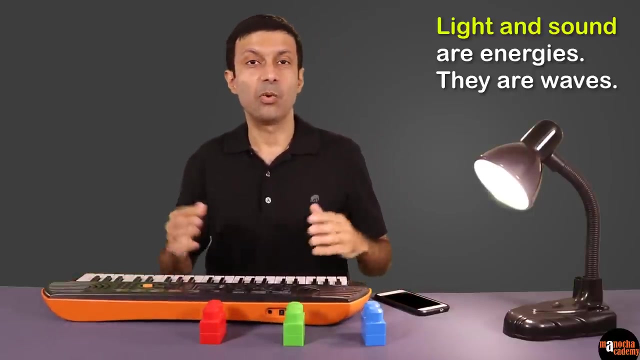 Now an interesting question is: why does light have different colors? So what is the difference between red light, green light or blue light? Let's compare light with sound. Light and sound are both energies, They are waves. So when I play music in this keyboard, 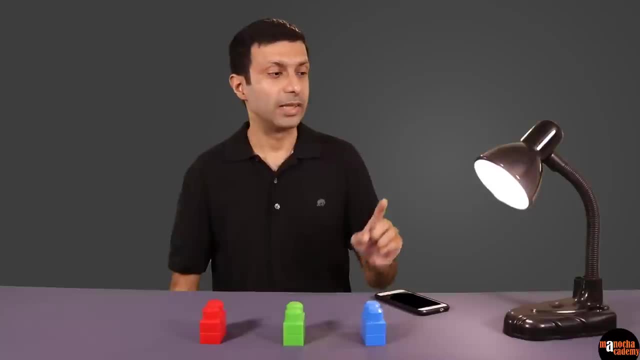 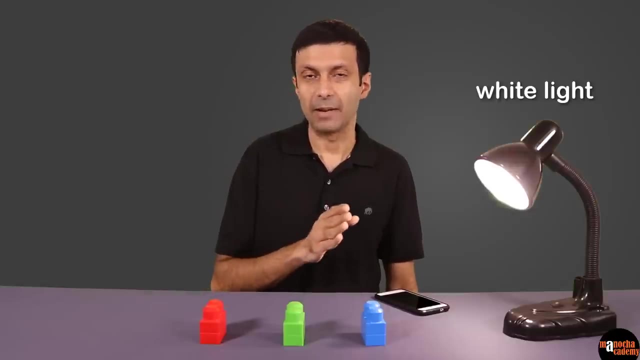 When we look at these three blocks under white light- whether it's coming from this bulb or from the lights in this room- we can see all the three colors: red, green and blue. The red block is reflecting red light. The green block reflects green light. 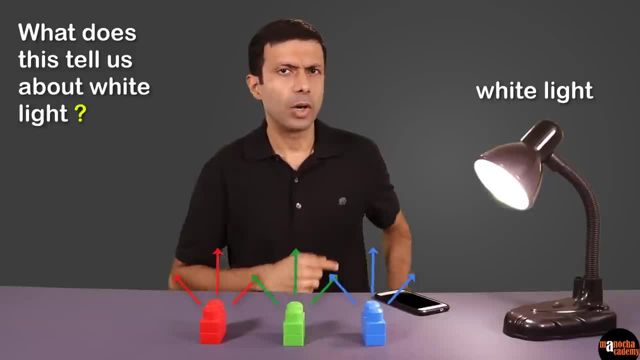 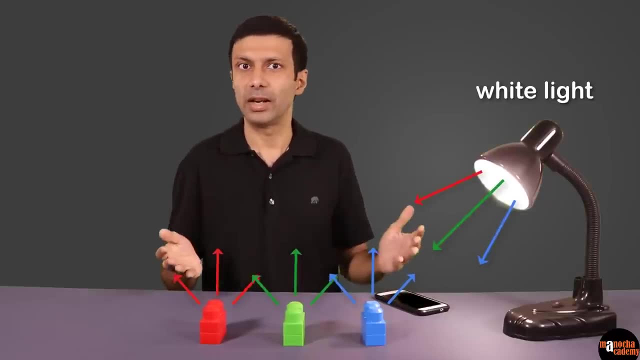 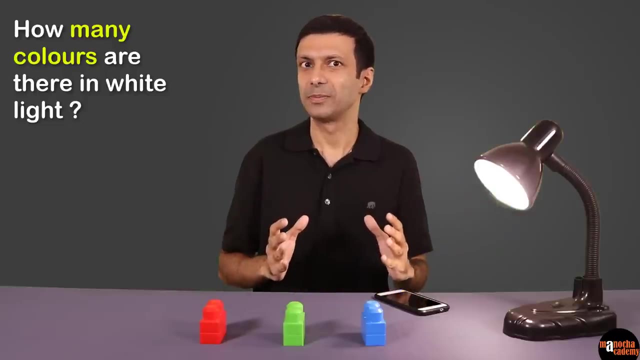 And the blue block reflects blue light. So what does this tell us about white light? White light is actually not white. It at least contains these three colors: red, green and blue. But do you know how many colors there are actually in white light? 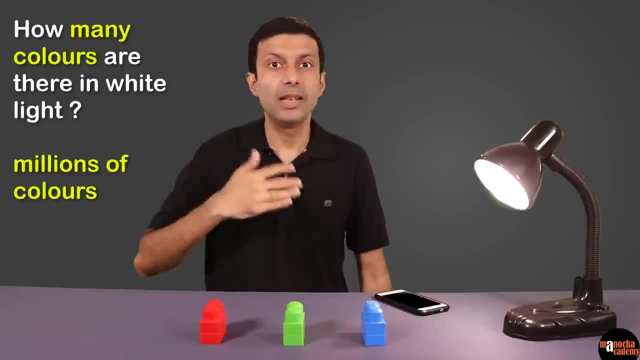 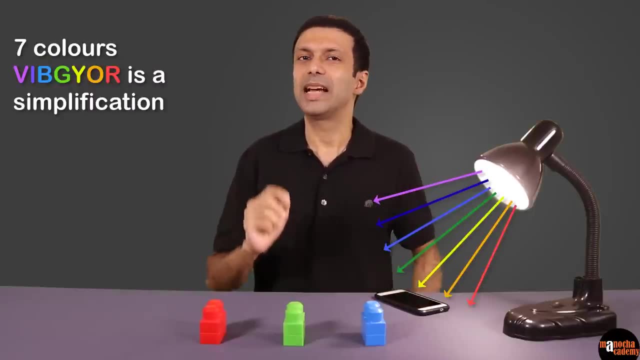 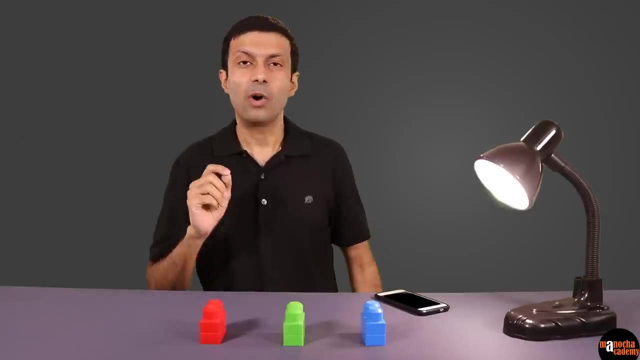 That's right. The correct answer is: white light contains millions and millions of colors. You may have heard of the seven rainbow colors or the Vibhgir colors, but that's just a simplification. White light is made up of three colors. White light is made up of millions and millions of colors. 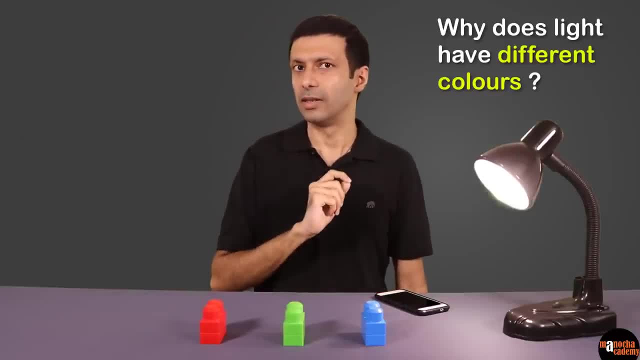 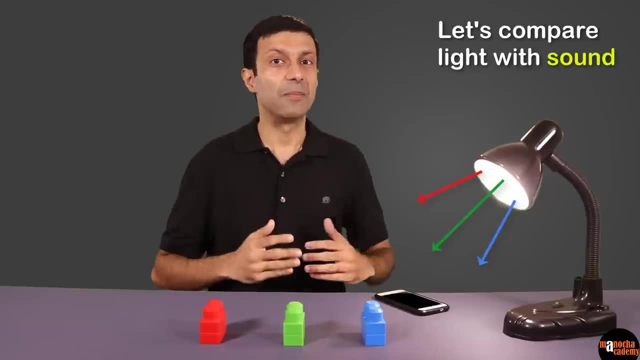 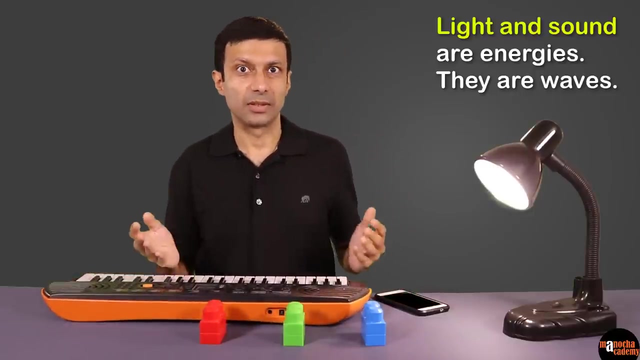 Now an interesting question is: why does light have different colors? So what is the difference between red light, green light or blue light? Let's compare light with sound. Light and sound are both energies, They are waves. So when I play music in this keyboard, why do these sounds sound different? 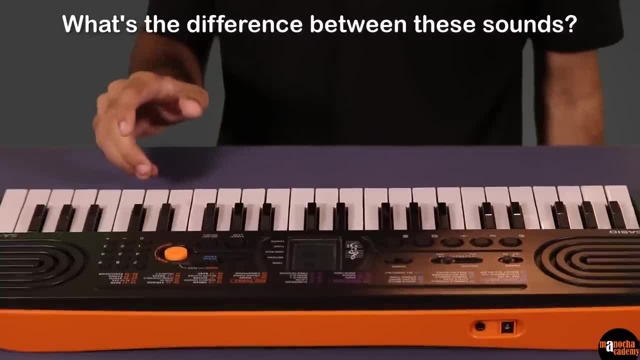 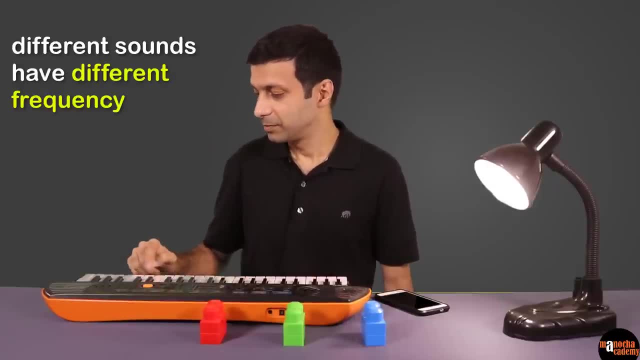 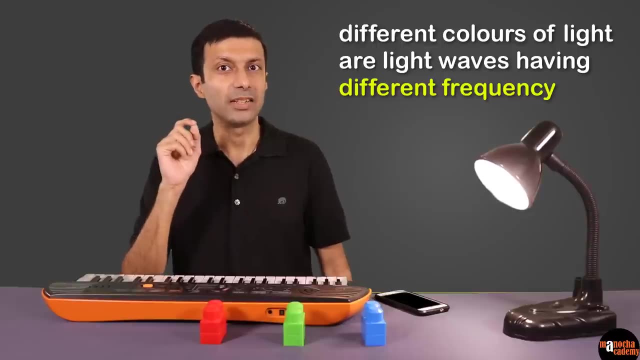 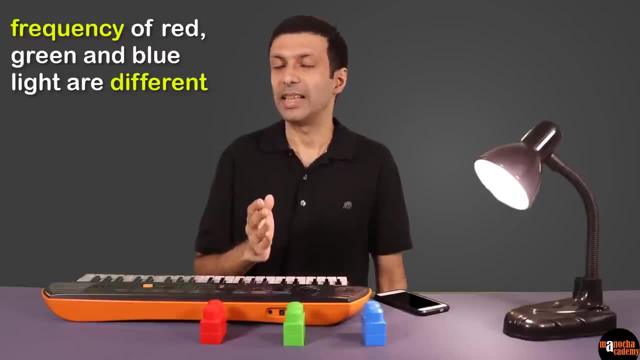 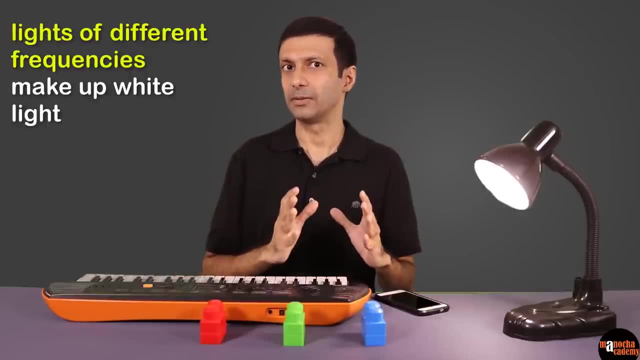 So the frequency of red light is different from green light and that's different from blue light, And all these light waves of different frequencies make up white light. Now can we separate the colors of white light Absolutely? Let's take a look how. 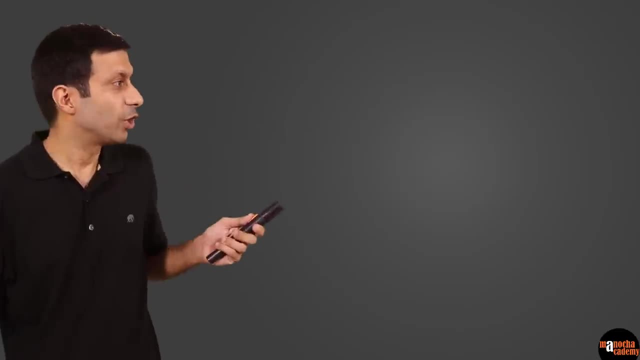 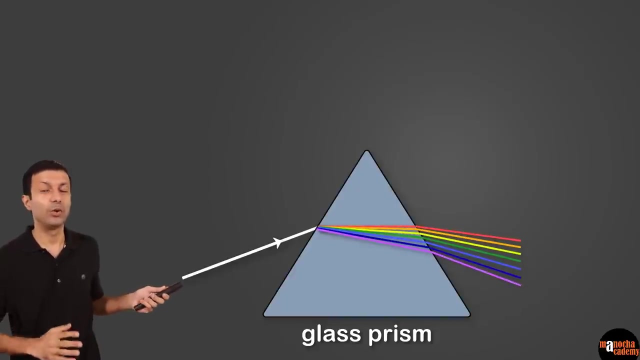 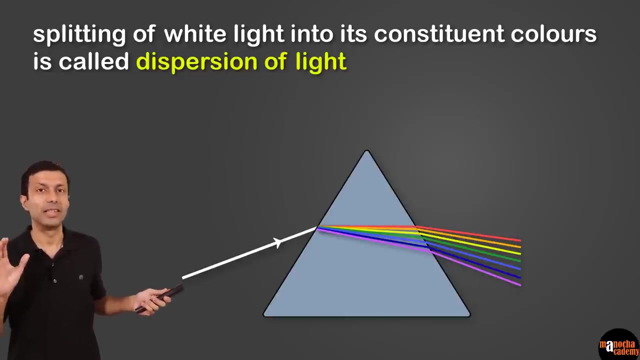 When you shine white light on a glass prism. as you can see, the glass prism splits white light into its constituent colors, And this splitting of white light into its constituent colors is called dispersion of light, And the band of colors obtained by this dispersion of light is called spectrum. 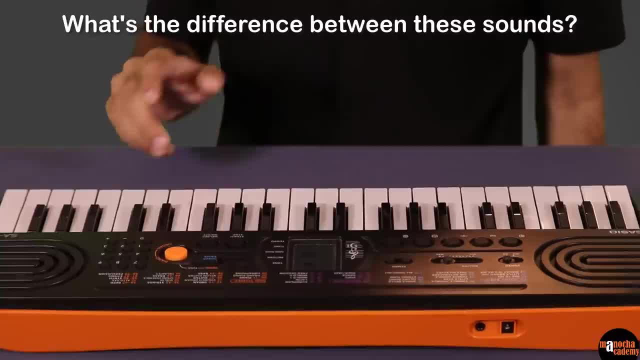 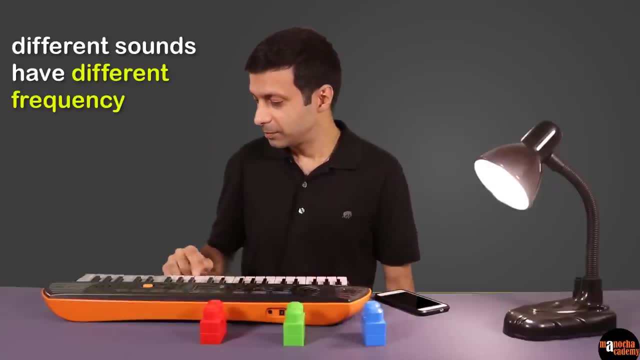 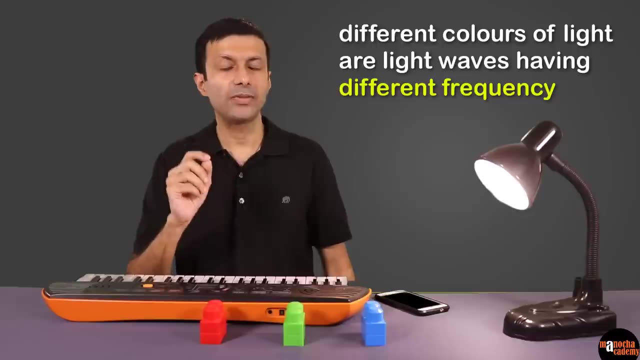 why do these sounds sound different? What's the difference between these sounds? That's right. these different sounds have different frequency. Similarly, different colors of light are light waves having different frequency. So the frequency of red light is different from green light. 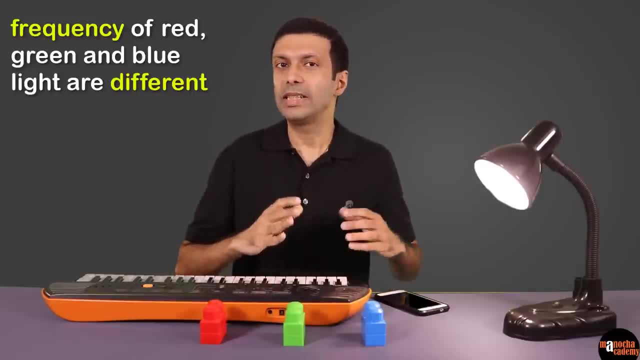 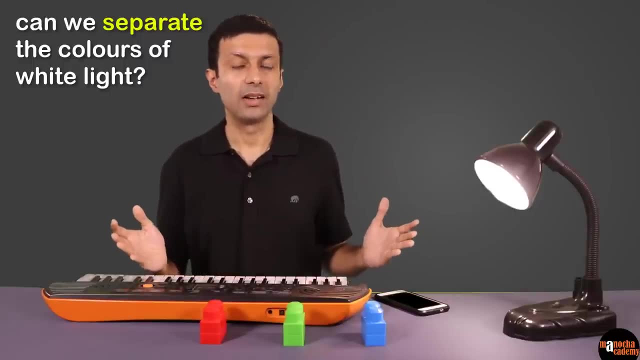 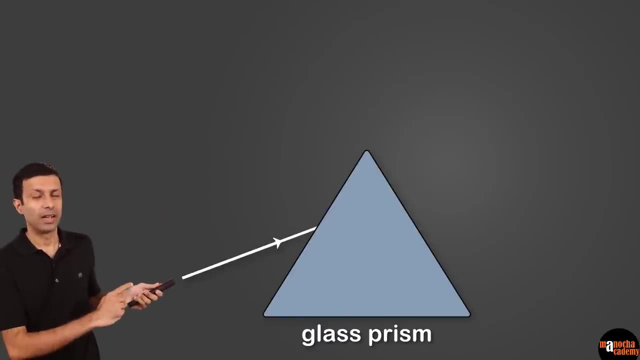 and that's different from blue light. And all these light waves of different frequencies make up white light. Now can we separate the colors of white light Absolutely? Let's take a look how, When you shine white light on a glass prism, as you can see, the glass prism splits the white light into its constituent colors. 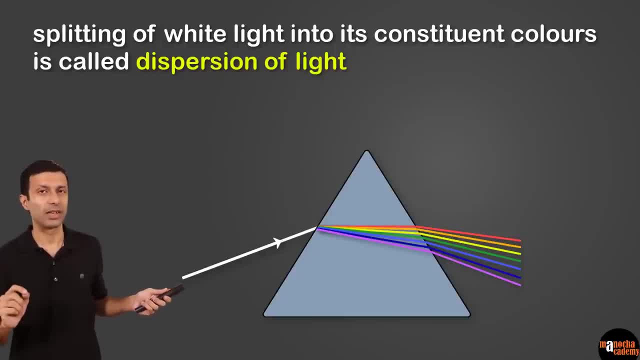 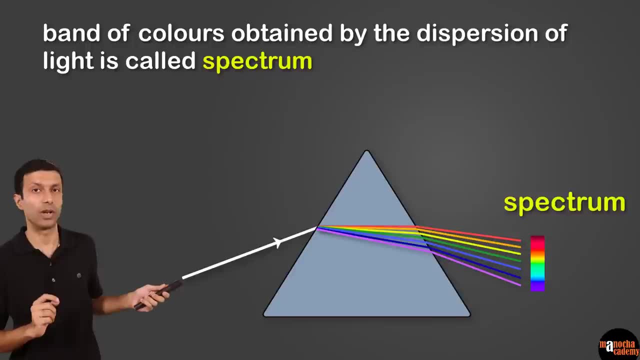 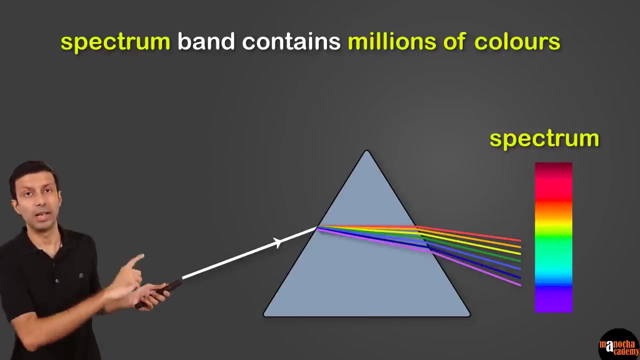 And this splitting of white light into its constituent colors is called dispersion of light, And the band of colors obtained by this dispersion of light is called spectrum. As we discussed, the spectrum band contains millions and millions of colors, But here we've just shown the seven rainbow colors. 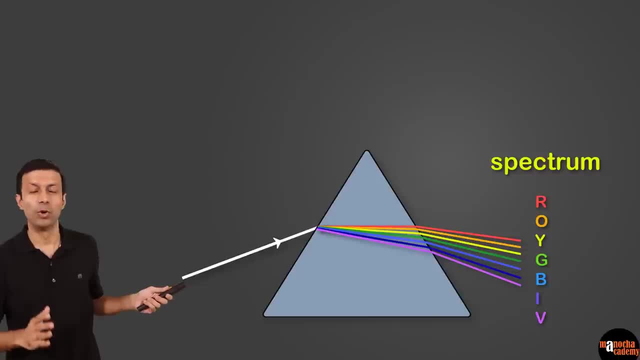 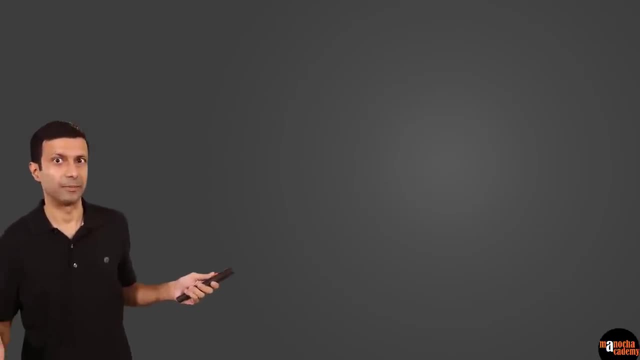 the Vibgir colors violet, indigo, blue, green, yellow, orange and red, just for simplicity. But actually there are millions and millions of colors there. Now can you think of examples where you've seen a spectrum, where you've seen the dispersion of light? 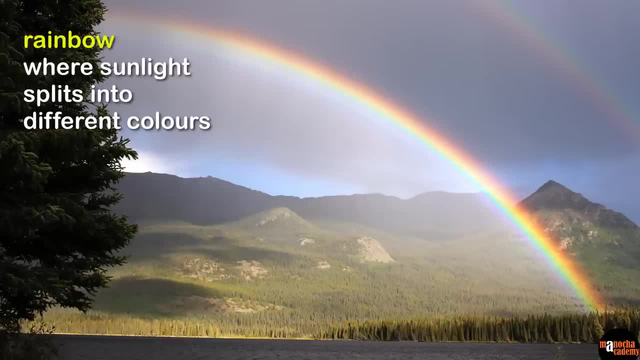 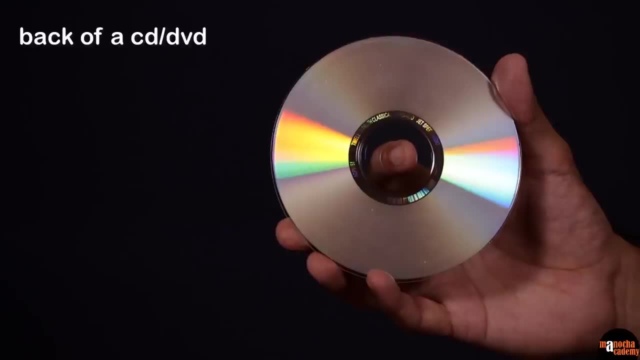 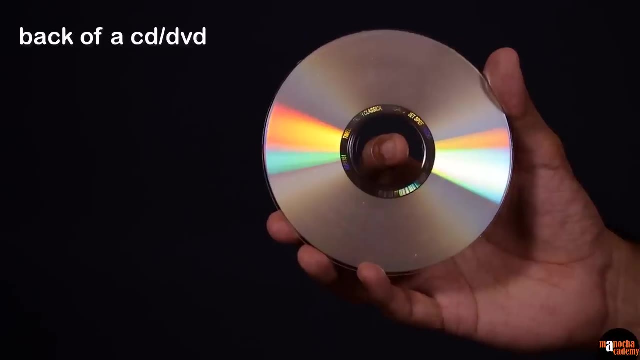 One simple example is the beautiful rainbow where you see the white sunlight splitting into the different colors. And another everyday life example is if you look at the back of a CD or DVD, have you seen the different colors? It looks almost like a rainbow. 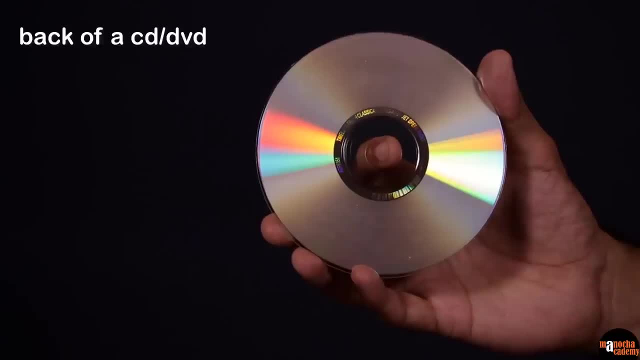 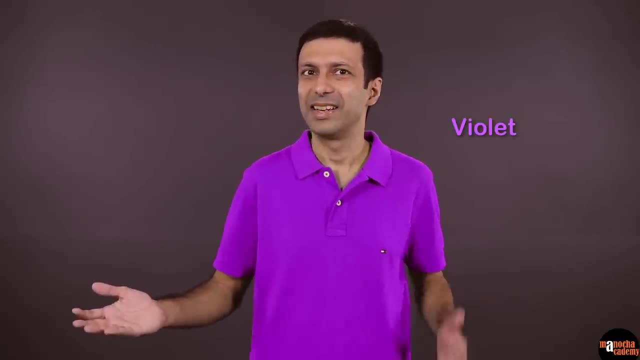 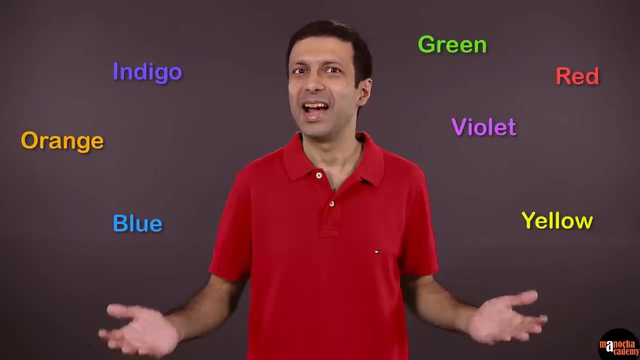 That's your spectrum, and it's happening due to dispersion of light. As we learnt, white light is made of seven different colors: Violet, indigo, blue, green, yellow, orange and red. This band of seven colors is known as spectrum. 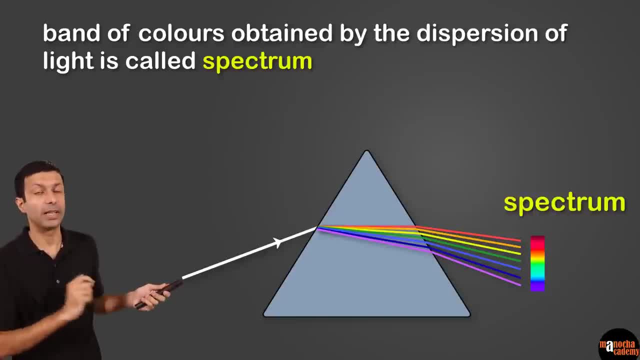 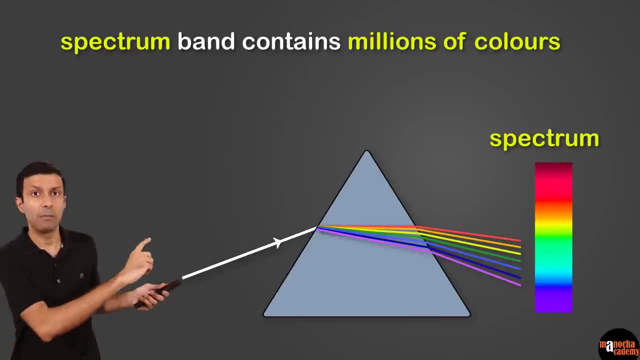 As we discussed, the spectrum band of spectrum light is called white light. White light is the band of spectrum light. White light is the band of spectrum light. the spectrum band contains millions and millions of colors, But here we've just shown the seven rainbow colors. 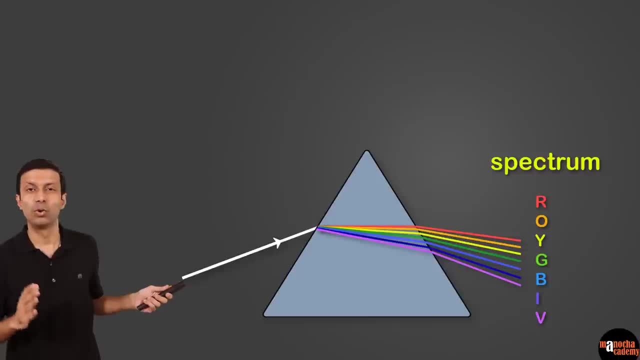 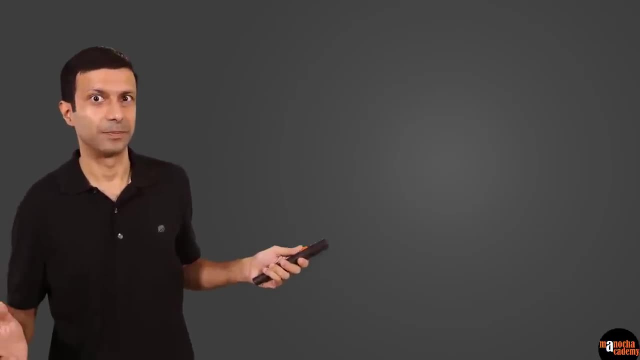 the Vibgir colors violet, indigo, blue, green, yellow, orange and red, just for simplicity. But actually there are millions and millions of colors there. Now can you think of examples where you've seen a spectrum? 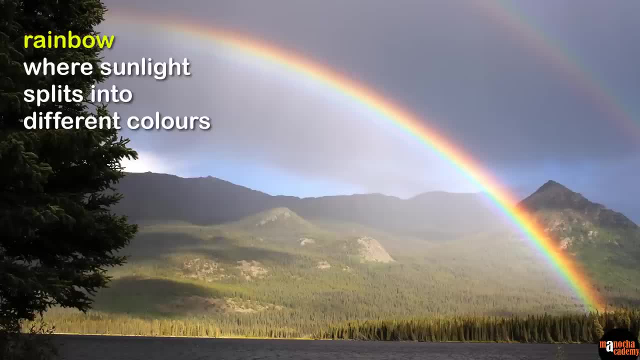 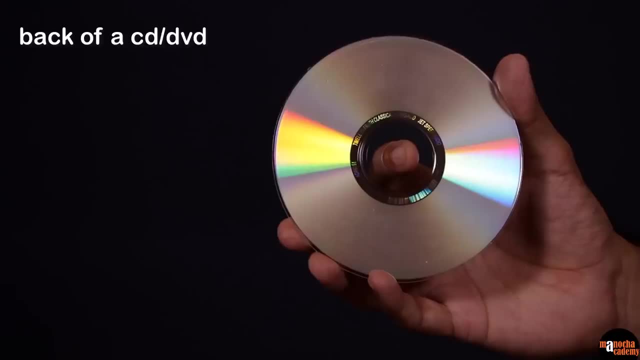 where you've seen the dispersion of light. One simple example is the beautiful rainbow, where you see the white sunlight splitting into the different colors. And another everyday life example is if you look at the back of a CD or DVD, have you seen the different colors? 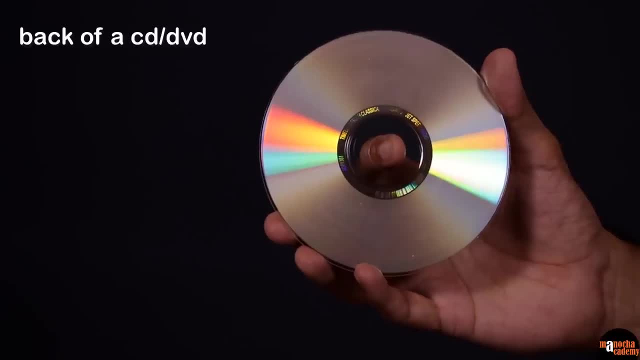 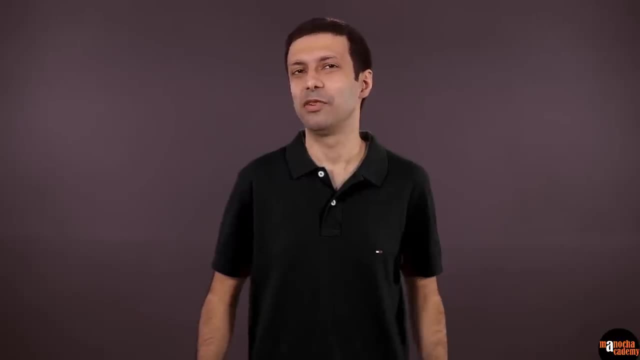 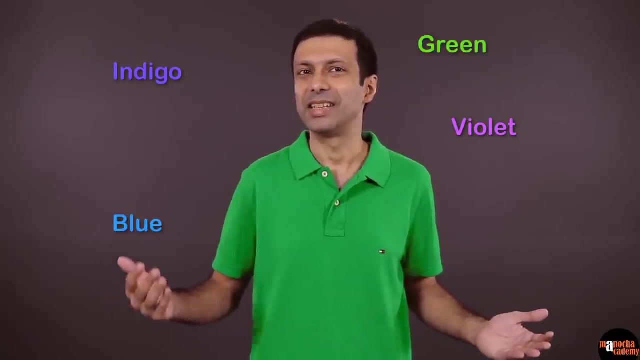 It looks almost like a rainbow. That's your spectrum and it's happening due to dispersion of light. As we learned, white light is made of seven different colors: Violet, indigo, blue, green, yellow, orange and red. 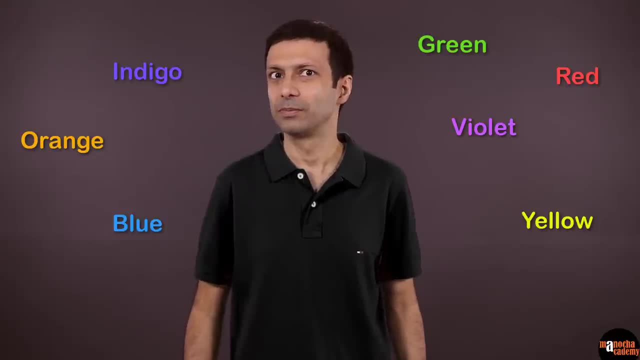 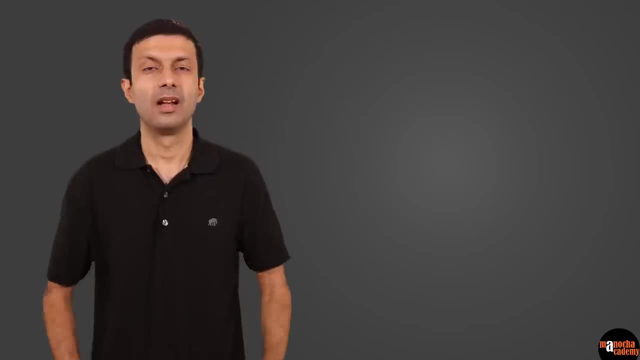 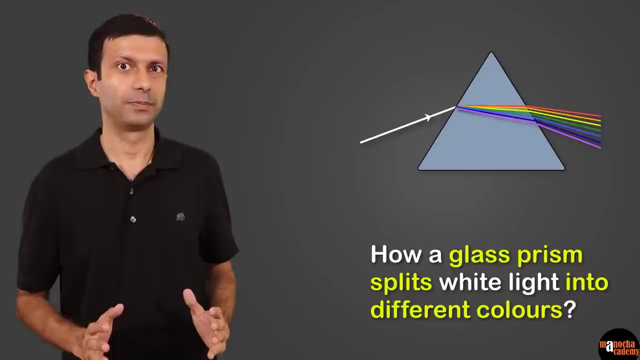 This band of seven colors is known as spectrum, And the splitting of white light into its constituent colors is known as dispersion of light. Now let's understand how a simple glass prism is able to split the white light into different colors. For this we need the concept of refraction. 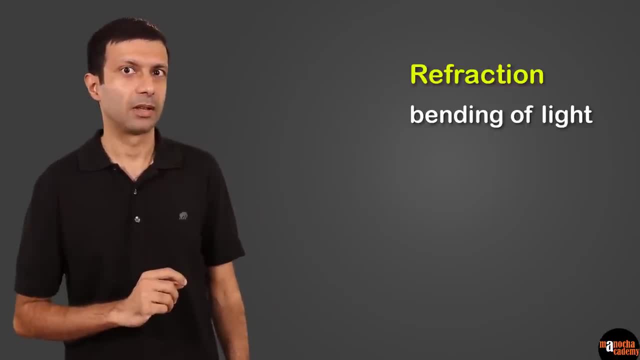 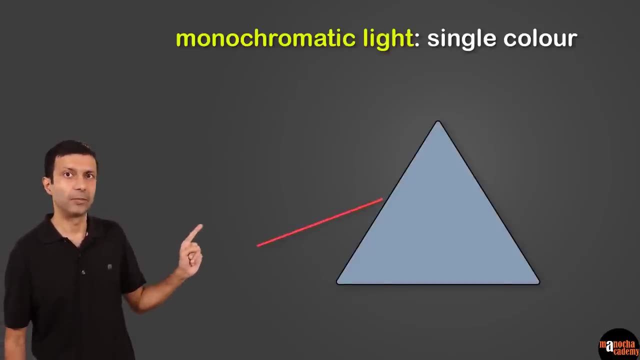 Remember, refraction means bending of light. So let's start off by shining light of a single color, known as monochromatic light, let's say red light here onto our glass prism And, as you can see, the light is traveling from air to glass. 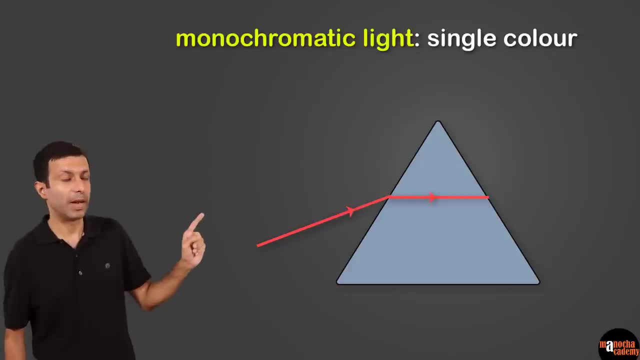 So there's a bending or refraction there And once again there's a bending when light comes out of the prism. so, from glass to air And, as you can see, the red light is bending towards the base of the prism here. 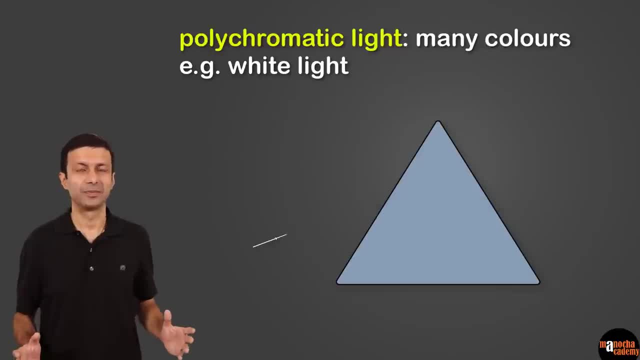 Now let's replace the red light with white light. Again, for simplicity, we'll consider that white light is made up of the seven Vibgior colors. Now, one important point to remember is that different colors of light have the same speed in air. 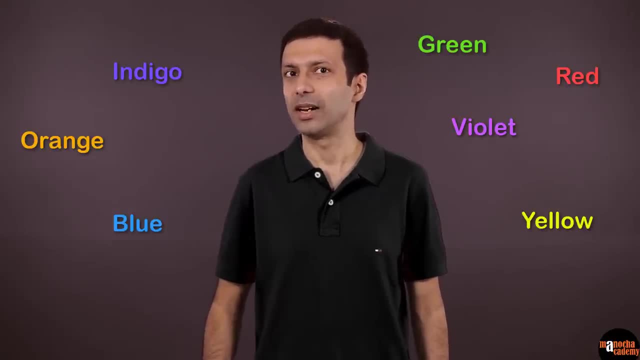 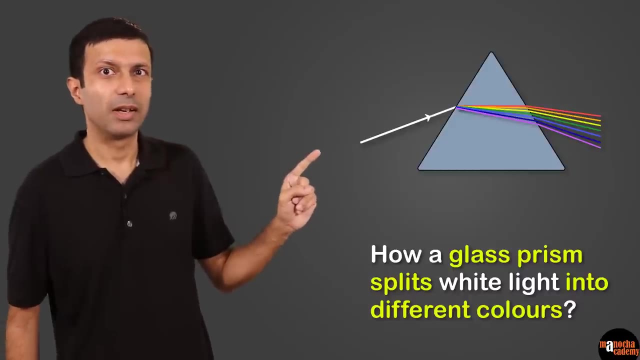 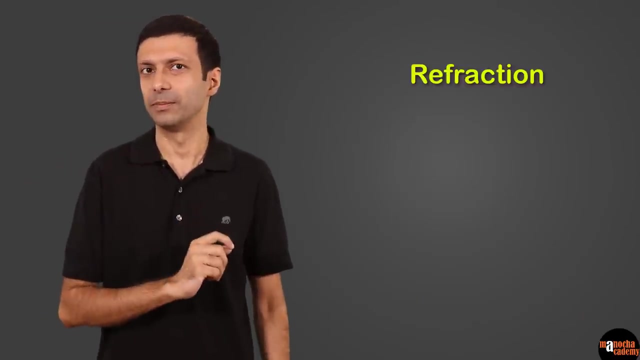 And the splitting of white light into its constituent colors is known as dispersion of light. Now let's understand how a simple glass prism is able to split the white light into different colors. For this we need the concept of refraction. Remember, refraction means bending of light. 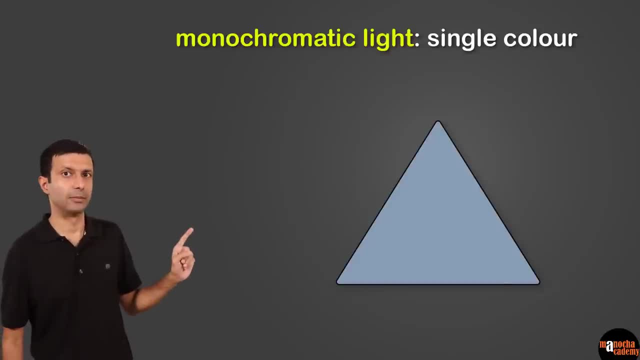 So let's start off by shining light of a single color, known as monochromatic light, let's say red light, here onto our glass prism And, as you can see, the light is traveling from air to glass, so there's a bending or refraction there. 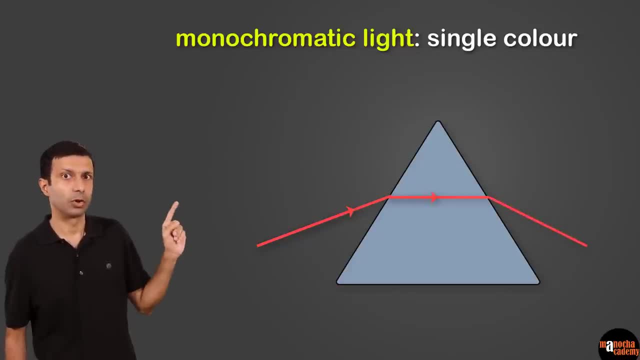 And once again, there's a bending when light comes out of the prism. so, from glass to air And, as you can see, the red light is bending towards the base of the prism. here Now let's replace the red light with white light. 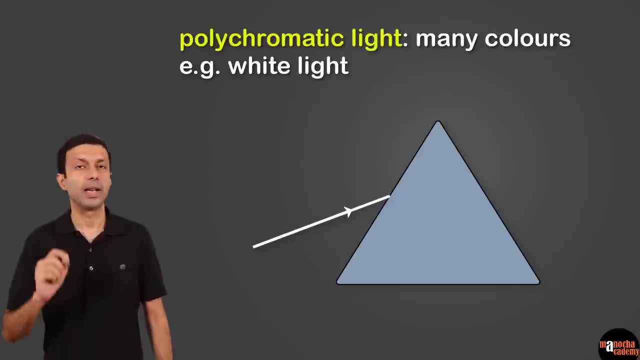 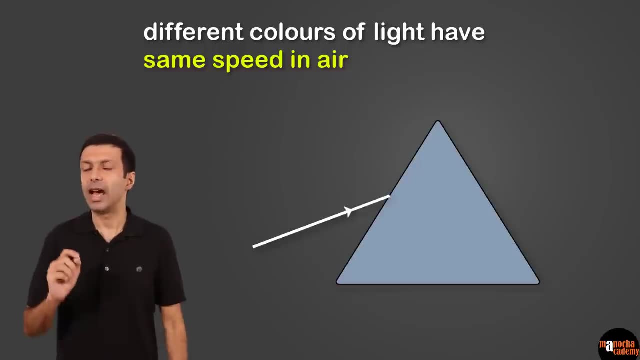 Again, for simplicity, we'll consider that white light is made up of the seven Vibgior colors. Now, one important point to remember is that different colors of light have the same speed in air, approximately 3 x 10 to the power, 8 meter per second. 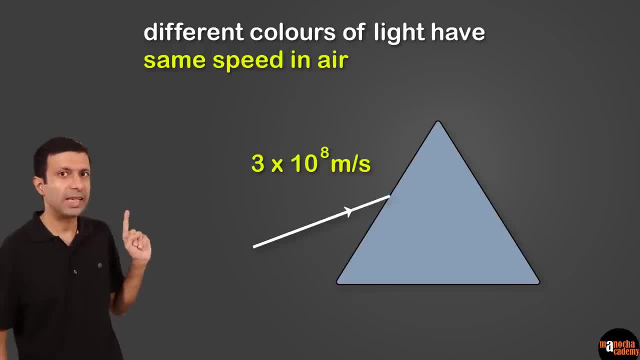 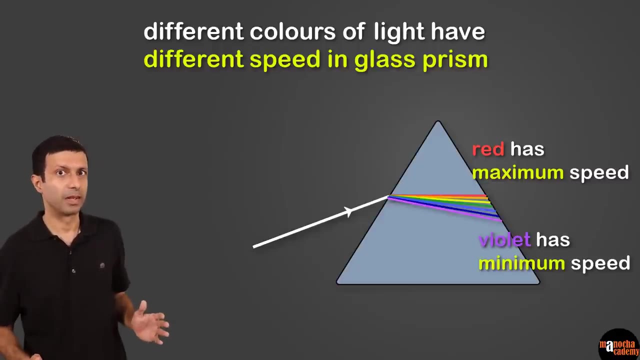 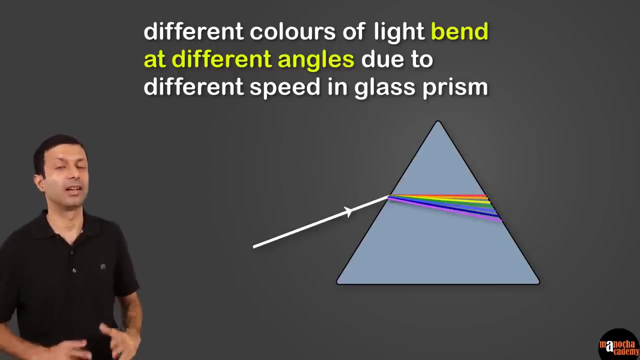 So all our seven colors are traveling at the same speed in air, But the moment they hit the glass prism, the speed of the different colors changes. in the glass prism, Red has the maximum speed and violet has the minimum speed. So because of the change in speed of the different colors, they bend at different angles in the glass prism. 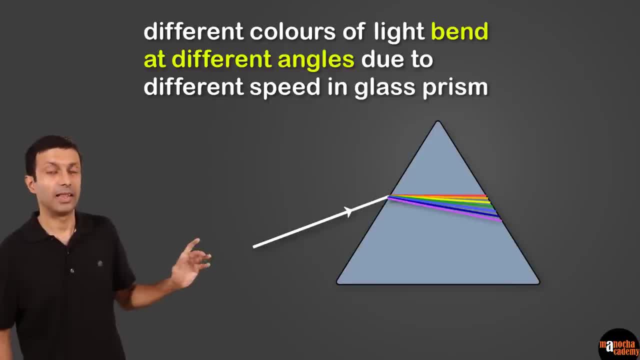 So, as you can see, they split there, And then there is another refraction when these different colors are coming out from the glass to the air. So this is how the glass prism is able to split the white light into its constituent colors. So the important point to remember is: all the colors have the same speed in air. 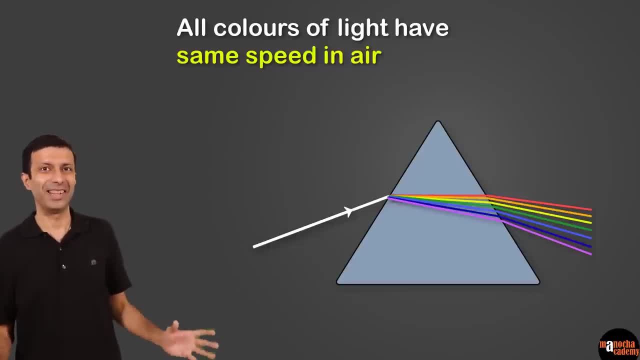 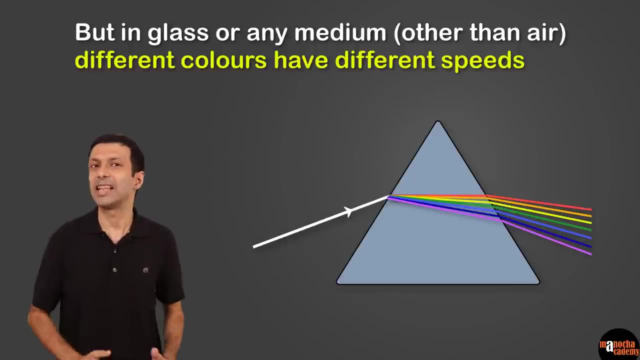 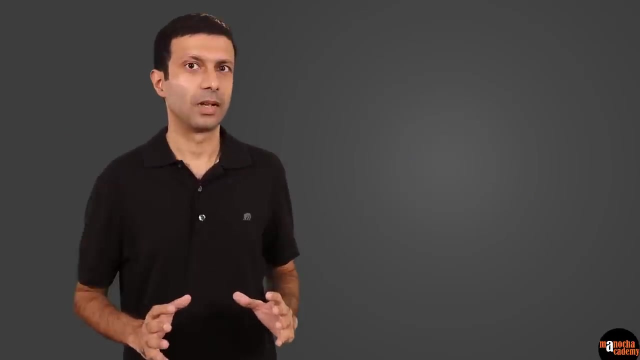 Otherwise we'll be seeing a rainbow right here in the air. But in glass or in any other medium, different colors have different speeds And that's how they split up. As we saw, our glass prism splits the white light into seven different colors. 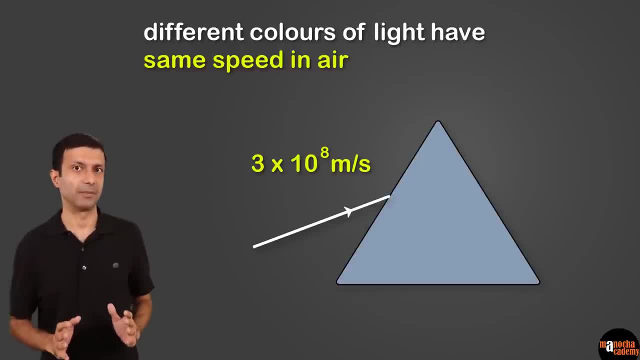 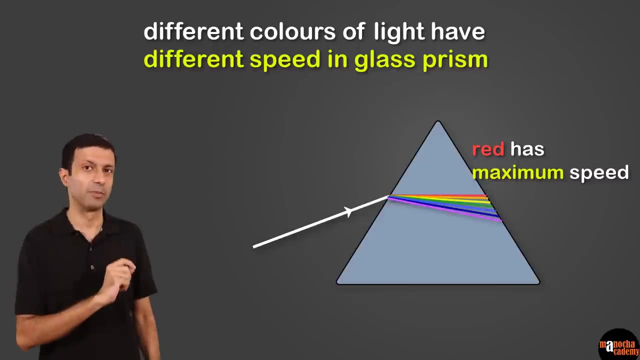 approximately 3 into 10 to the power, 8 meter per second. So all our seven colors are traveling at the same speed in air, But the moment they hit the glass prism, the speed of the different colors changes. in the glass prism, Red has the maximum speed and violet has the minimum speed. 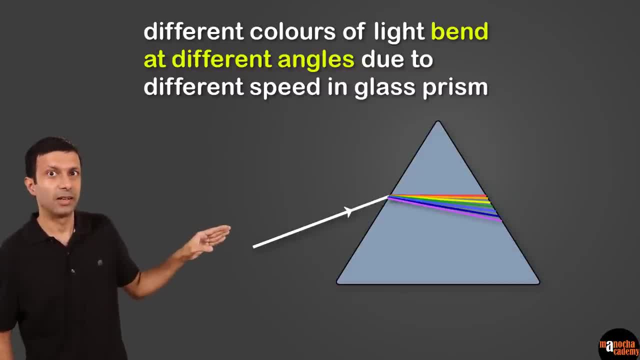 So, because of the change in speed of the different colors, they bend at different angles in the glass prism So, as you can see, they split there, And then there is another refraction when these different colors are coming out from the glass to the air. 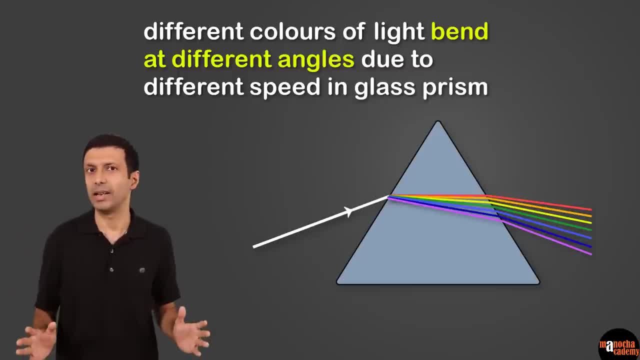 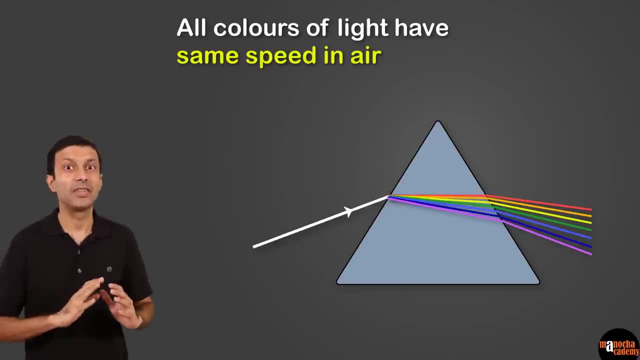 So this is how the glass prism is able to split the white light into two parts. So the glass prism is able to split the white light into its constituent colors. So the important point to remember is: all the colors have the same speed in air. 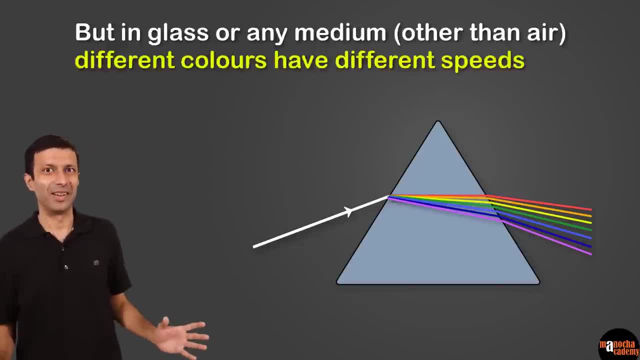 Otherwise we'll be seeing a rainbow right here in the air. But in glass or in any other medium, different colors have different speeds and that's how they split up. As we saw, our glass prism splits the white light into seven different colors. 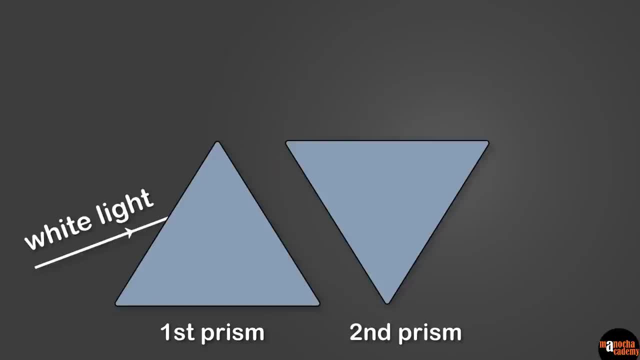 Now what do you think is going to happen if we place a second prism on top of the first one, But it's inverted after the first one. That's right, We are going to get back white light again. So these two prisms are showing that white light contains seven colors. 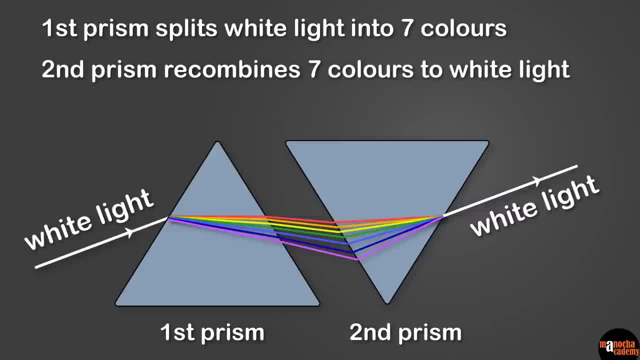 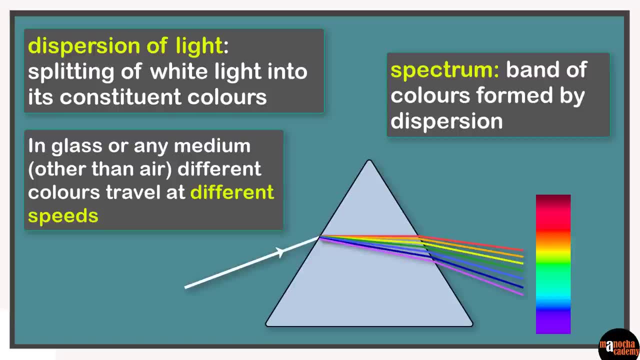 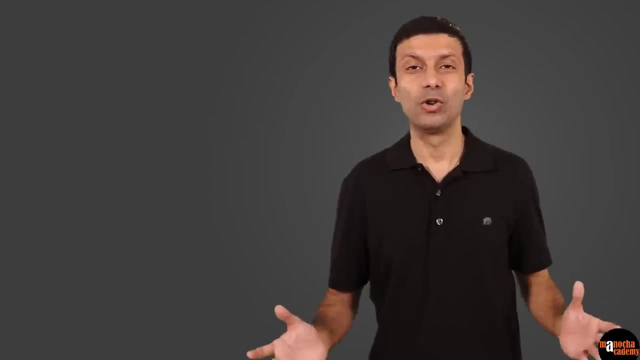 The first one is splitting the white light into seven colors, and the second prism recombines the seven different colors back to white light. Let's place the concepts we have learned so far on our concept board. Now let's talk about nature's beautiful spectrum: the rainbow. 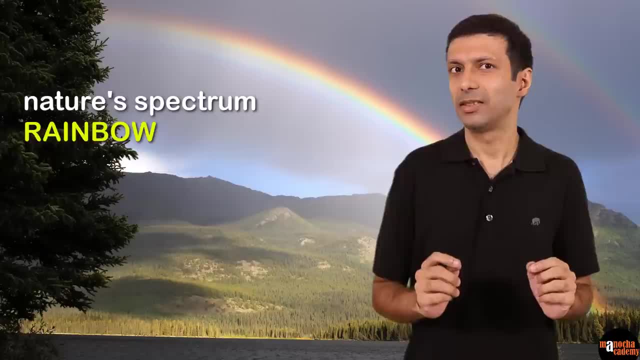 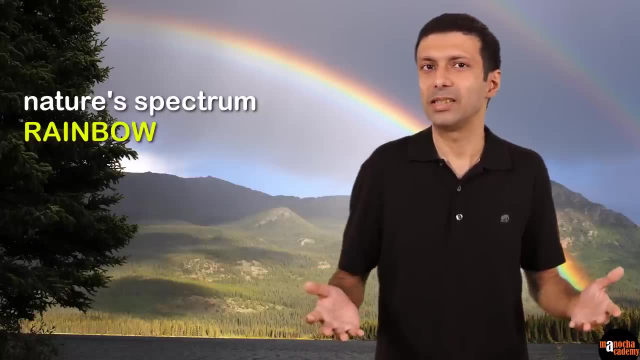 I'm sure you've seen a rainbow, but it's pretty rare, right, Because you need both rainfall and sunshine happening at the same time and it only lasts a few seconds or a few minutes. But can you think of some places where you'll always see a natural rainbow? 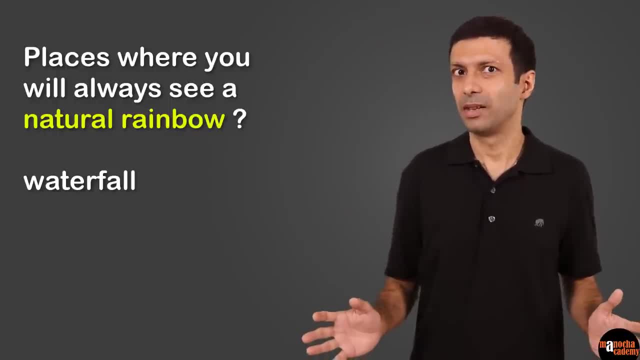 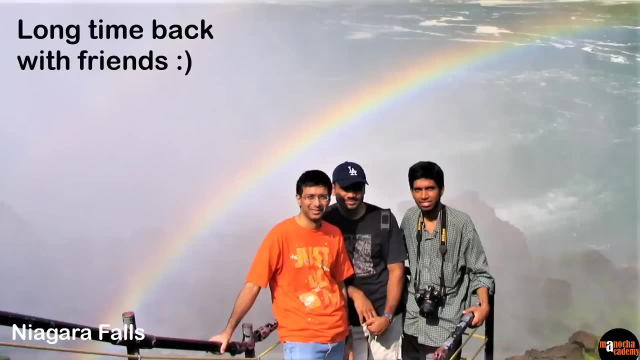 One thing that comes to my mind is near a waterfall. I've been to the Niagara Falls, where you'll always see a rainbow. It never disappears and people are clicking pictures around that rainbow. Let's discuss how a rainfall rainbow is formed. 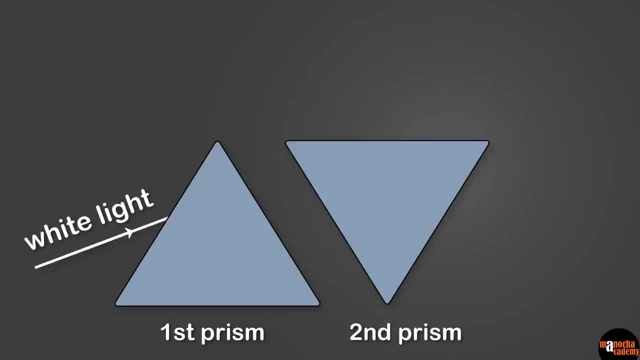 Now what do you think is going to happen if we place a second prism but it's inverted after the first one. That's right, We are going to get back white light again. So these two prisms are showing that white light contains seven colors. 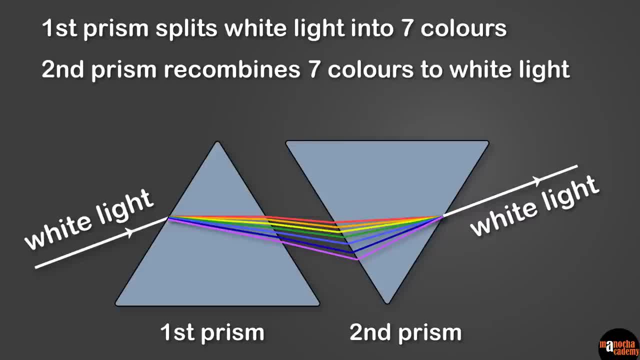 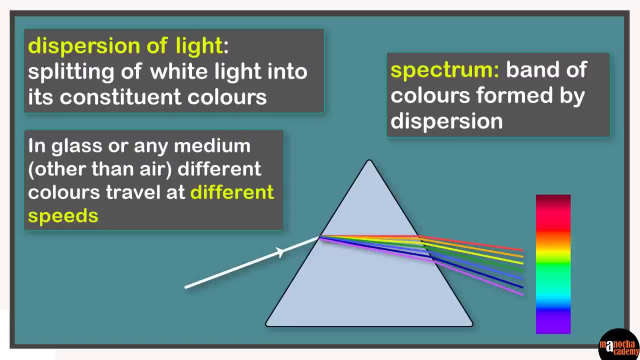 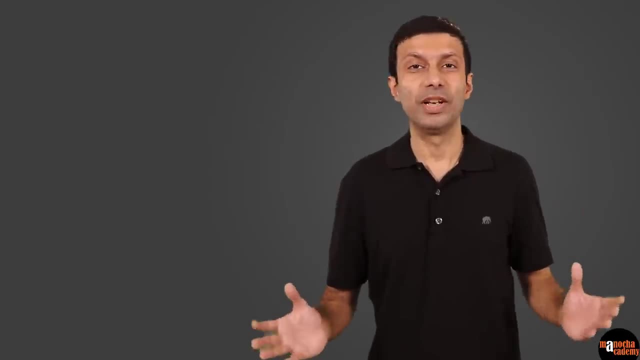 The first one is splitting the white light into seven colors, and the second prism recombines the seven different colors back to white light. Let's place the concepts we have learned so far on our concept board. Now let's talk about nature's beautiful spectrum: the rainbow. 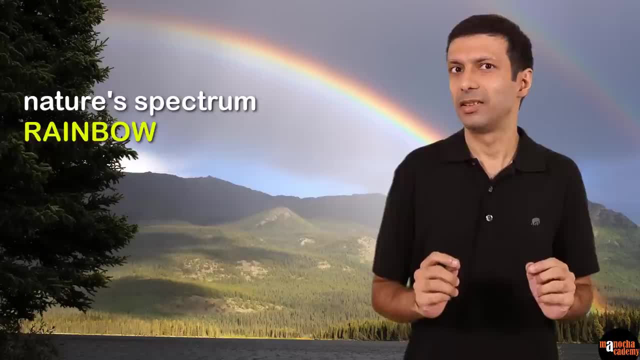 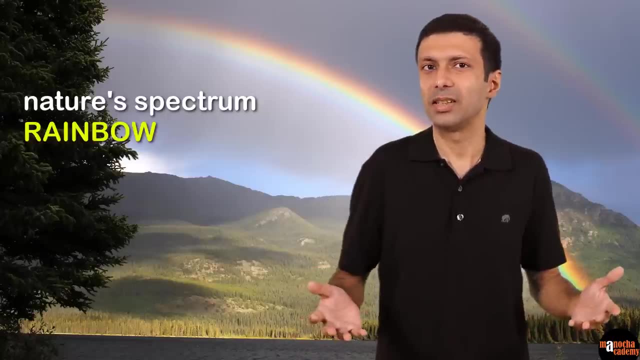 I'm sure you've seen a rainbow, but it's pretty rare, right, Because you need both rainfall and sunshine happening at the same time And it only lasts a few seconds or a few minutes. But can you think of some places where you'll always see a natural rainbow? 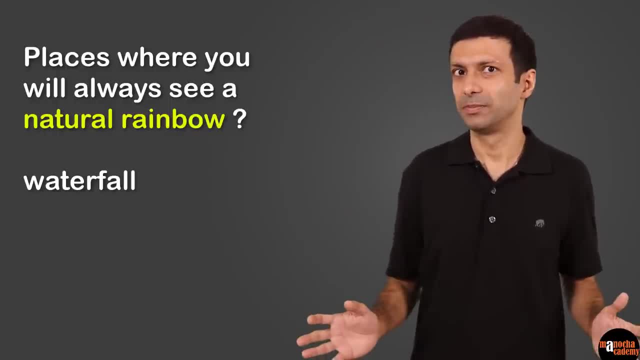 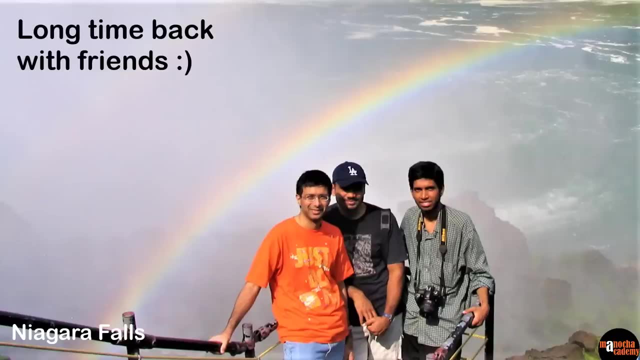 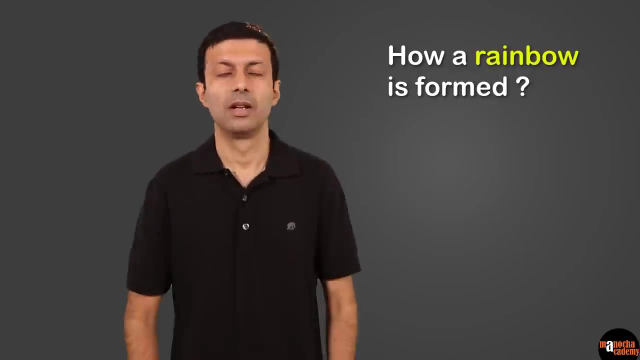 One thing that comes to my mind is: near a waterfall. I've been to the Niagara Falls and there you'll always see a rainbow. It never disappears and people are clicking pictures around that rainbow. Let's discuss how a rainfall rainbow is formed. 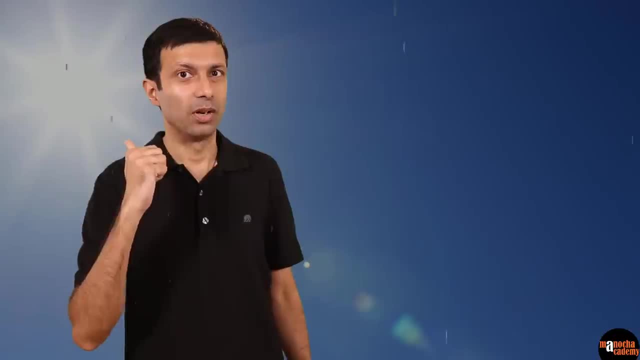 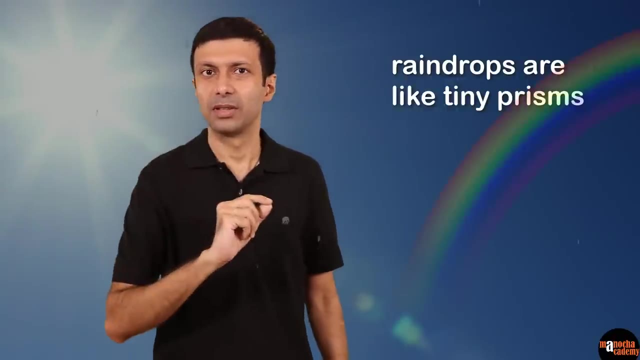 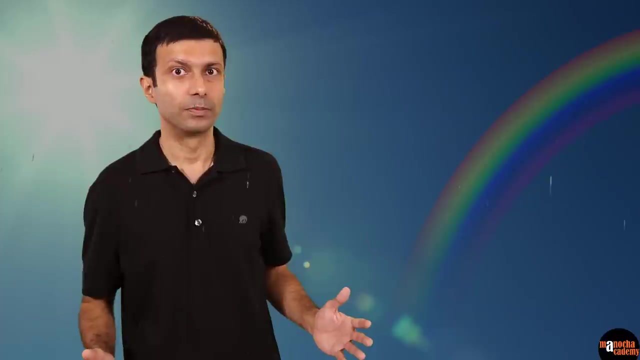 To see the rainbow, you need the sun behind you and you need to be looking towards the rain. The raindrops are acting like tiny, tiny prisms and they are splitting the white light of the sun into the seven different colors forming our rainbow. 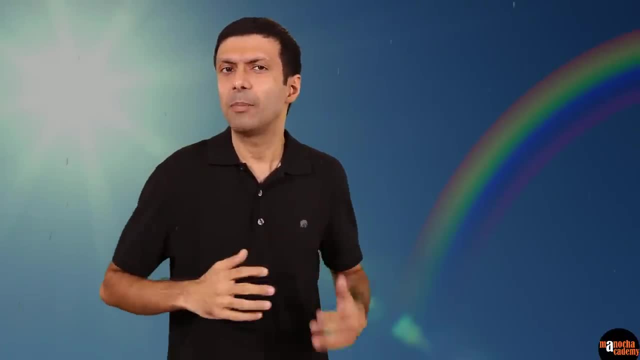 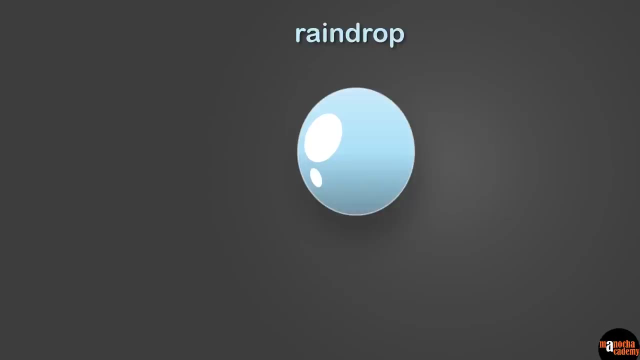 But it's not just dispersion of light involved. There's some other stuff going on. Let's take a closer look. Let's consider one raindrop for simplicity. When the white light from the sun enters the raindrop, just like the prism, it splits into seven colors. 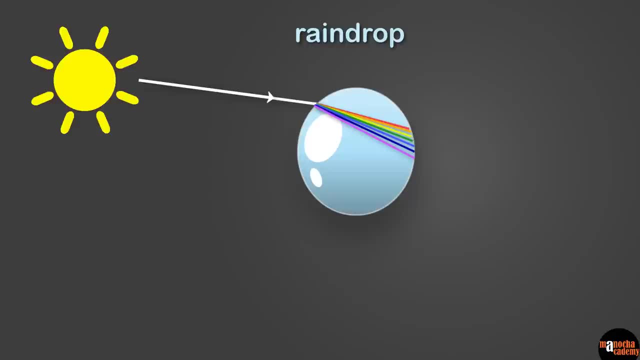 Because light is entering from air to water in the raindrop, And we know that different colors of light will have different speeds in water, So there's dispersion there Now, rather than all the colors of the light leaving the raindrop, an interesting thing happens, which is known as total internal reflection of light. 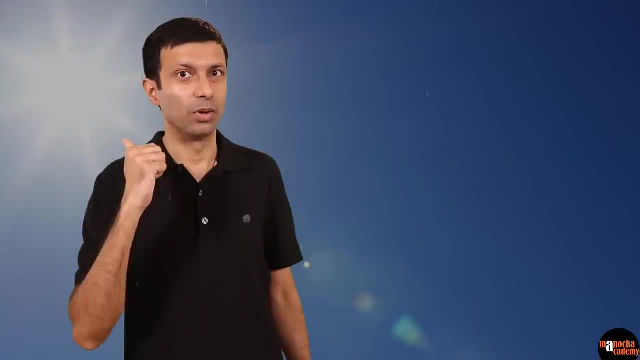 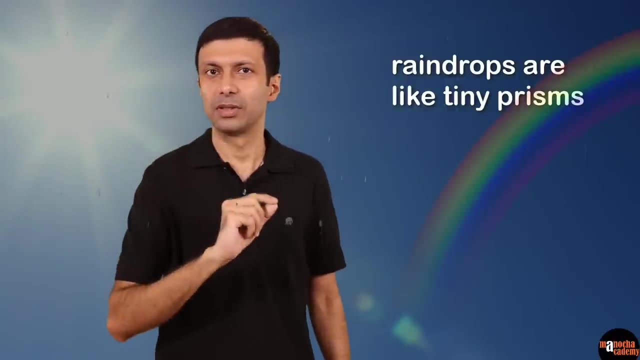 To see the rainbow, you need the sun behind you and you need to be looking towards the rain. The raindrops are acting like tiny, tiny prisms and they are splitting the white light of the sun into the seven different colors forming our rainbow. 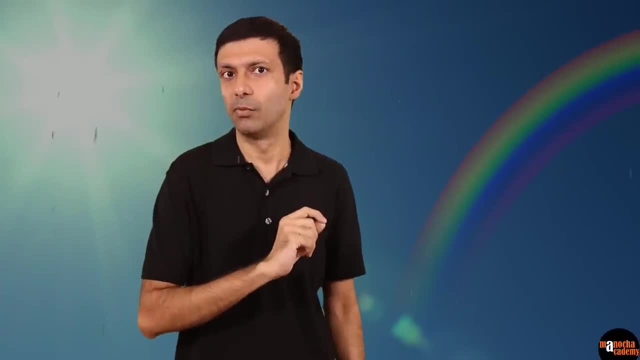 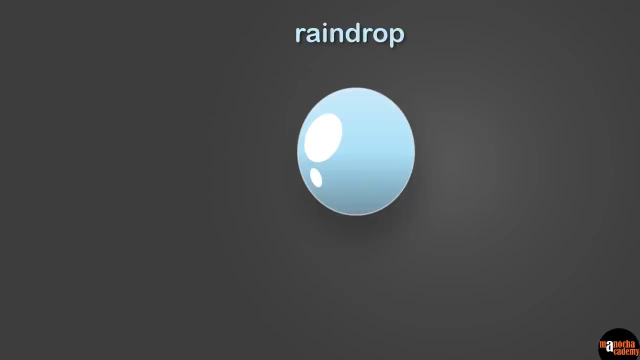 But it's not just dispersion of light involved. there's some other stuff going on. Let's take a closer look. Let's consider one raindrop for simplicity. When the white light from the sun enters the raindrop, just like the prism, it splits into seven colors. 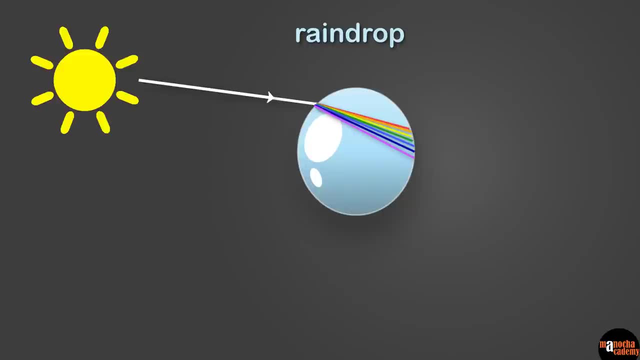 Because light is entering from air to water in the raindrop, and we know that different colors of light will have different speeds in water, So there's dispersion there Now, rather than all the colors of the light leaving the raindrop, an interesting thing happens, which is known as total internal reflection of light. 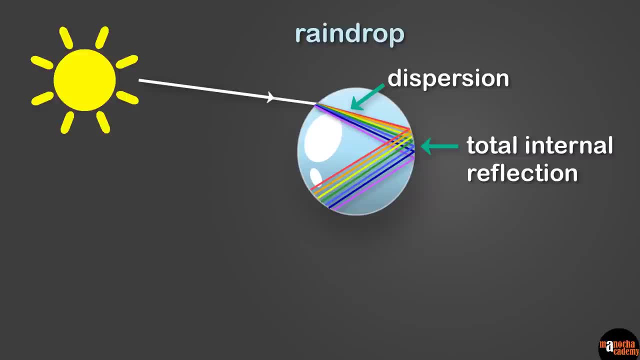 This takes place because light is traveling from a denser to a rarer medium, in this case from water to air, And the angle of incidence of light is greater than the critical angle of water. So instead of refracting all, the colors get reflected back. 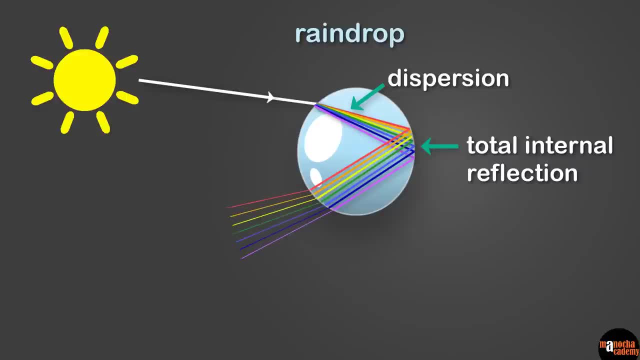 And now the seven colors. The seven colors again try to lead the raindrop. This time the angle of incidence is lesser than the critical angle, So there is refraction of light, And that's how we see the seven beautiful colors of the rainbow. 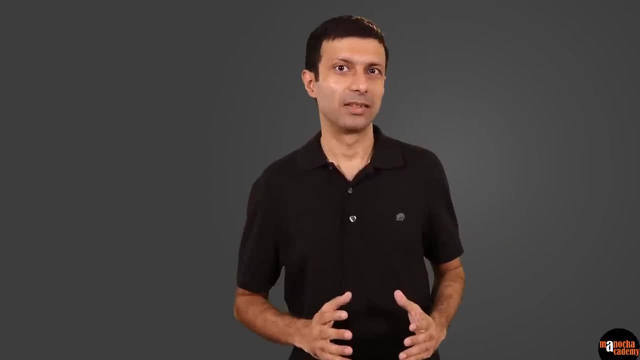 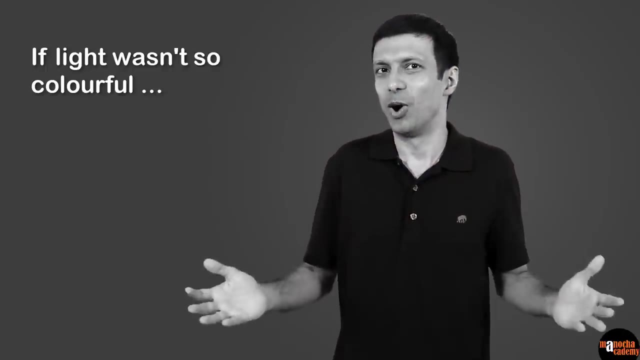 As we've learnt, light is made up of many different colors. But if light wasn't so colorful, it would be like watching an old black and white movie. But we don't want that right. So let's get the colors back on. 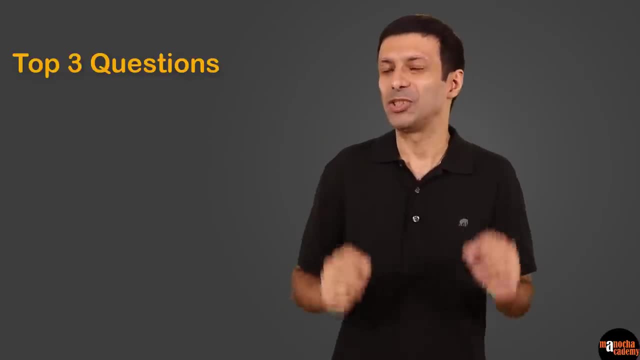 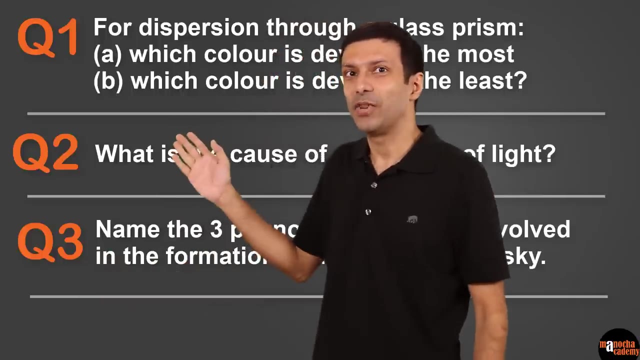 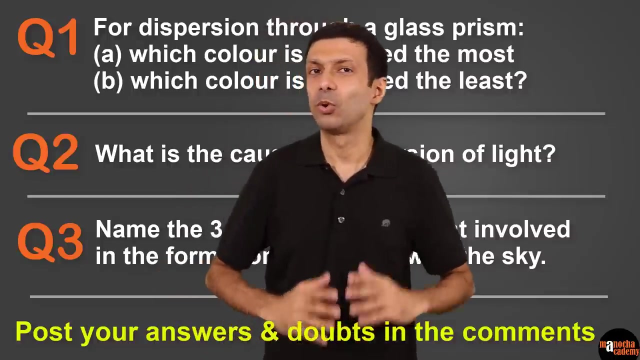 And now are you ready for the three questions on this topic coming up for you right now? Friends, try solving these questions and let me know your answers and doubts by putting it in the comments below. I promise to reply to all your comments as soon as possible. 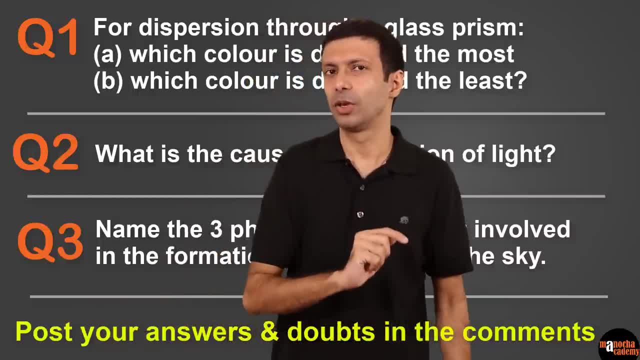 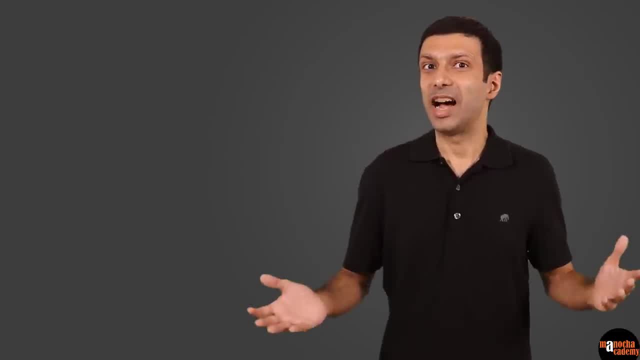 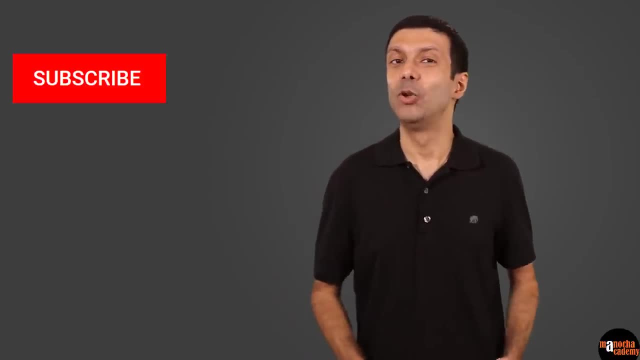 So I'm going to disappear and you pause the video here and give these questions a shot. Friends, I hope you enjoyed this colorful video, So do hit the red subscribe button for my YouTube channel and the blue like and follow button for my Facebook page.